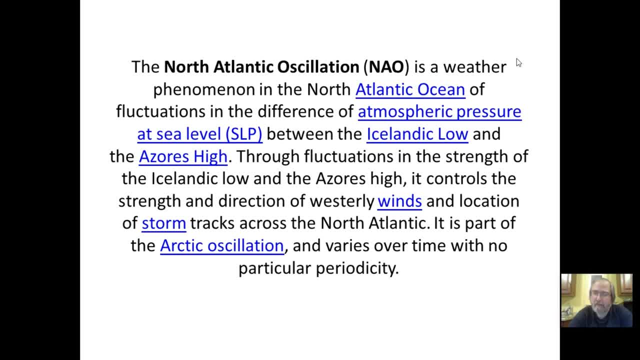 difference of atmospheric pressure at sea level, called SLP, sea level pressure between the Icelandic low and the Azores high. Through fluctuations in the strength of the Icelandic low and the Azores high, it controls the strength in direction of westerly winds and location of. 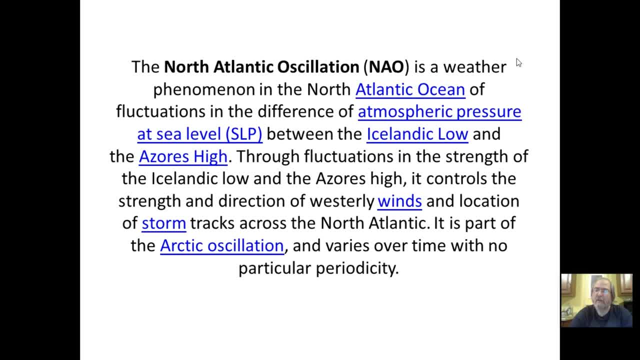 storm tracks across the North Atlantic. It is also part of the Arctic Oscillation and varies over time with no particular periodicity, which makes analyses a little more challenging. Now I've just completed a video of discussing gyras and rotating systems, so hopefully now you have a good handle when we start discussing that, because highs and 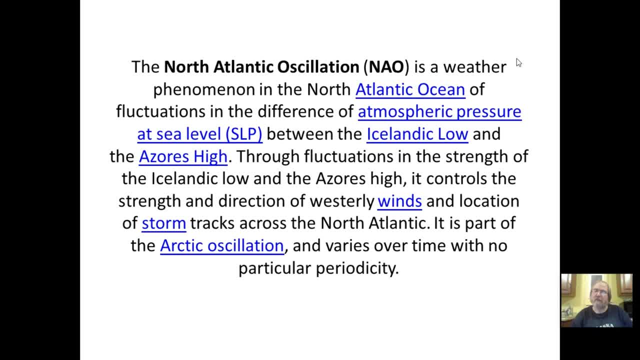 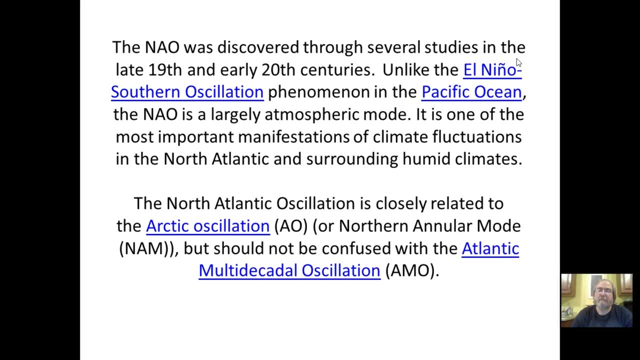 lows are going to really play a strong part when we look at the NAO, the Arctic Oscillation and the Atlantic Multi-Decadal Oscillation. So what's going on here? The NAO was discovered through several studies in the late 19th and early 20th centuries. 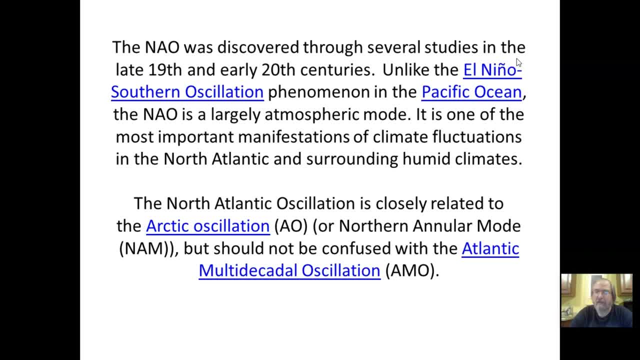 Unlike the ENSO, the El Nino Southern Oscillation Phenomenon in the Pacific Ocean, the NAO is a largely atmospheric mode. Okay, remember, in our discussion with ENSO, it was not only the atmosphere in the low pressure system but also what was going on with the ocean. 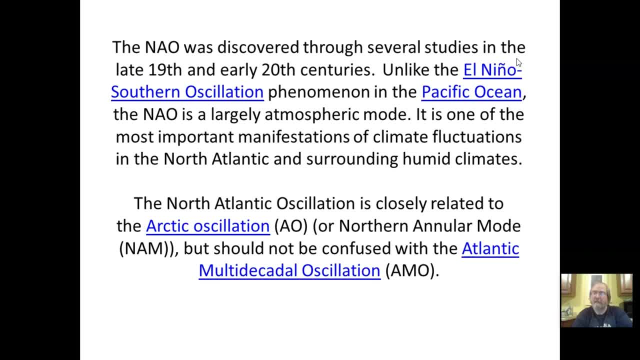 and how the atmosphere was impacting the ocean, like the fisheries- again the fisheries example- and just the flow of the water, how the water is piling up, etc. The NAO is more atmospheric but it's still going to impact the ocean. But, as we saw with ENSO, the ocean and 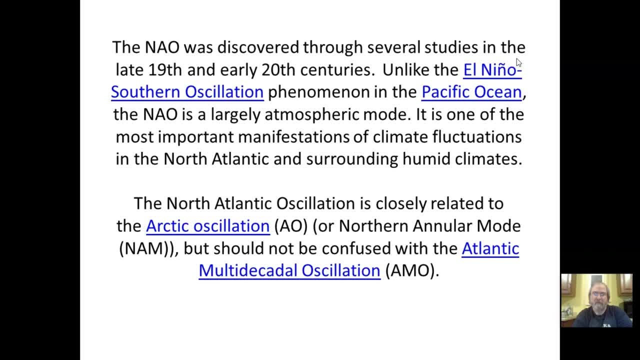 the atmosphere are really tightly tied together. Right Recall that when the wind blowing from east west are really strong pushes the water towards indonesia and australia. that allows the pycnocline to rise up on the eastern side with the upwelling and good for the fishery when winds reverse, or 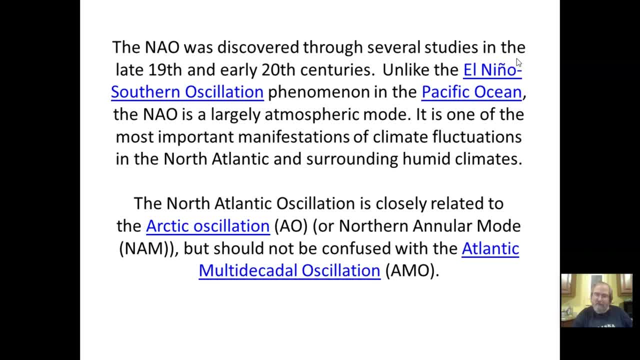 weaken, then all that water that piled up on the western side moves to the east. get that warm water blob moving to the east and then the pycnocline is depressed. instead of having an upwelling, you have a downwelling and the fisheries don't do as well. right, all all the tied in with the, the wind. 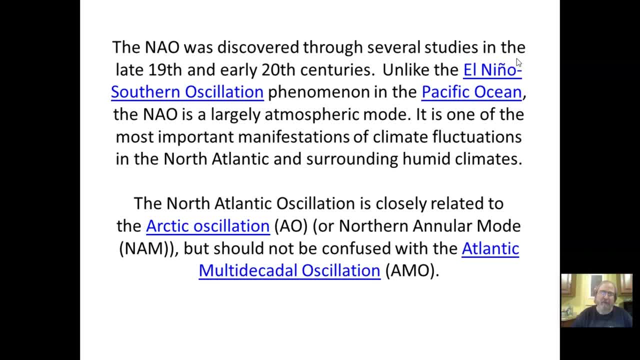 forcing, which is tied into the atmospheric system, the highs and the lows and how they're moving back and forth. and then, of course, we tied that all together with, uh, the ipo and, more so, the pdo. i consider the ipo and pdo to be kind of a, an integrated system, uh, but be that as it may, we 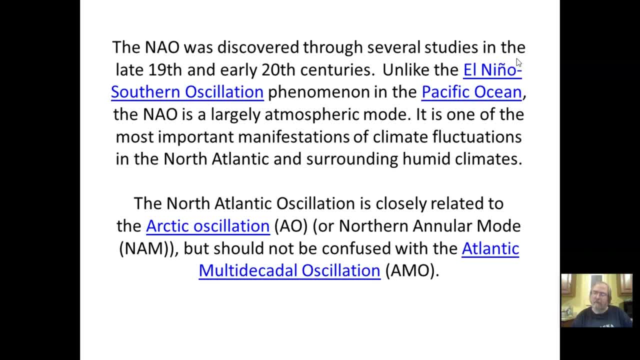 saw all that and, uh, i that was all discussed in prior videos. the north atlantic oscillation is closely related to the arctic oscillation, which is the ao, something that's called the northern annular mode. then you have the southern annular mode, which is basically antarctica but should not be confused with the atlantic. 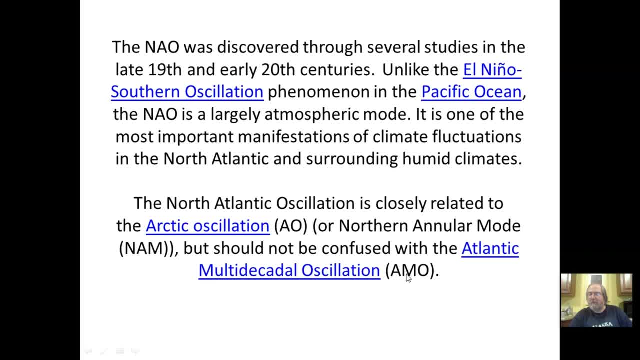 multi-decadal oscillation, or ammo. okay, it's funny because in latin uh, ammo means i love. that's interesting, but uh, you, so um, i will be doing a separate video of the arctic oscillation. i thought about doing both of these in one video, but it might be end up being very long-winded. there already are. 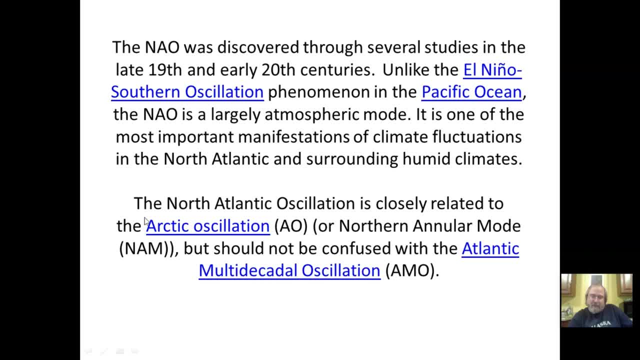 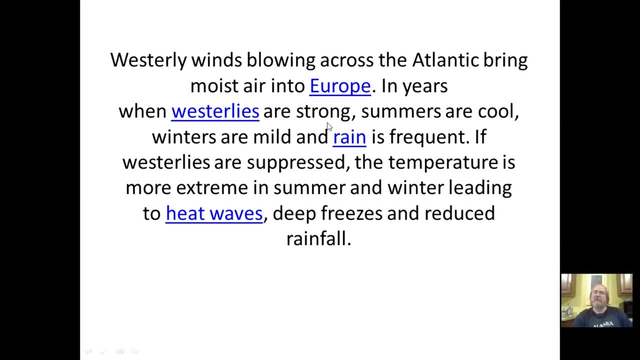 long-winded my videos on this stuff, so this will be a separate video, but it'll follow right after the nao and then that will in turn follow by the amo. westerly winds blowing across the atlantic bring moist air into europe. in years where westerlies are. 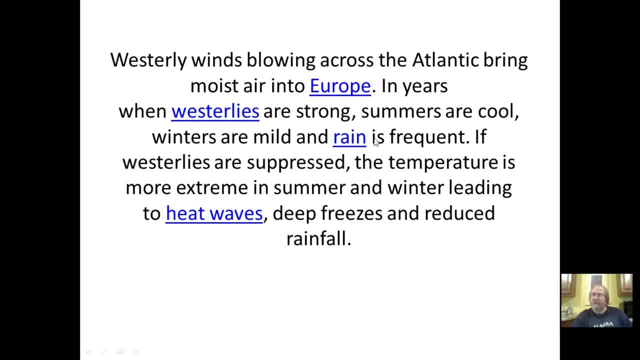 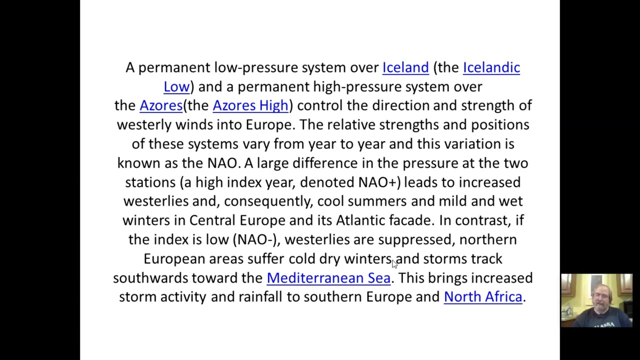 strong. summers are cool, which is a mild. rain is frequent- excuse me if the westerlies are suppressed. the temperature is more extreme in summer and winter, leading to heat waves, deep freezes and reduce rainfall or any precipitation, be that a permanent low pressure system over iceland, the icelandic low and a permanent high pressure. system over the azores. the azores high control the directions between南rwesel and zwel animals, between midwest and northwest. in 2017, the low high pressure westerly winds against steep Himalayan LGBT populations are alkaline. moist air Protocol 14 wave. 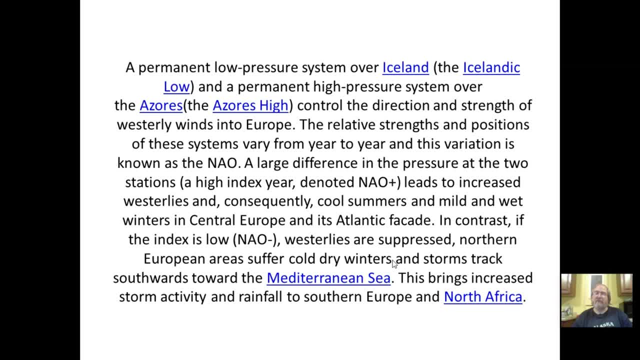 and least three- retour steam Far East portfolio 18 it is not a relative strength in候 he encuentra � theikat is low and a o negative wesley's are suppressed northern european areas suffer cold dry winters and storms track southwards towards the mediterranean sea this brings increased 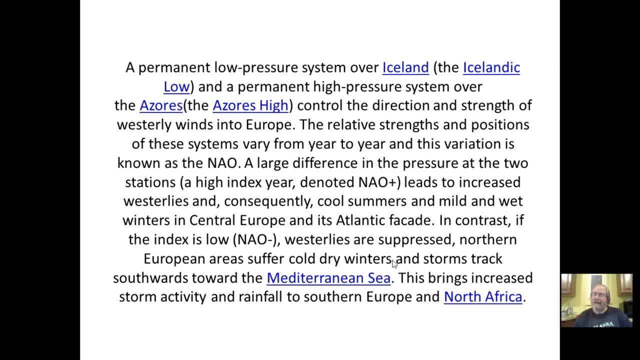 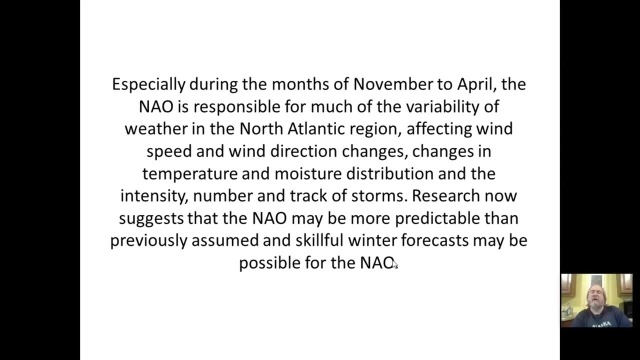 storm activity and rainfall to southern europe and north africa okay, especially during the months from november to april. the nao is responsible for much of the variability of weather in the north atlantic region, affecting wind speed, wind direction changes, changes in temperature, moisture distribution and the intensity, number and track of storms. research now suggests that. 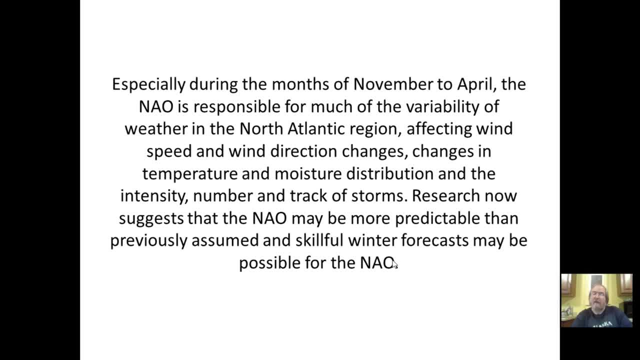 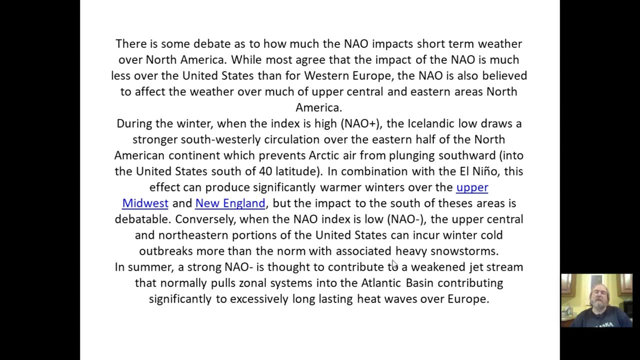 the nao may be more predictable than previously assumed, and skillful winter forecasts may be possible for the nao. like anything else, you collect more data. your understanding improves. that will enable us to predict better what happens in the future. there is some debate as to how much you can predict better what happens in the future. there is some debate as to how much. 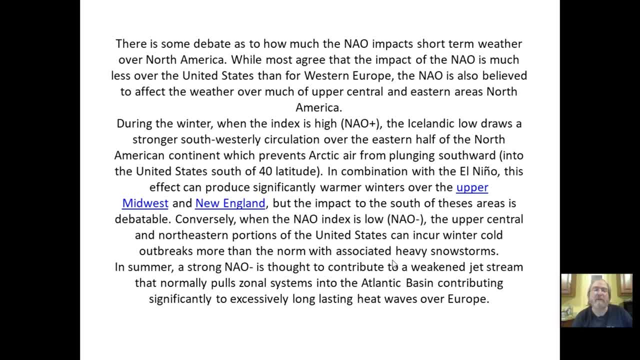 the nao impacts impact short-term weather over north america. while most agree the impact of the nao is much less over the us than for western europe, the nao is also believed to affect the weather over much of upper central eastern areas of north america, tied into the arctic oscillation. during the winter, when the index is high, the icelandic load draws a stronger southwestly circulation over the eastern half of the north american continent, which prevents arctic air from diving southward into the us south of 40 degrees latitude. in combination with el nino, this effect can produce significantly warmer winters over the. 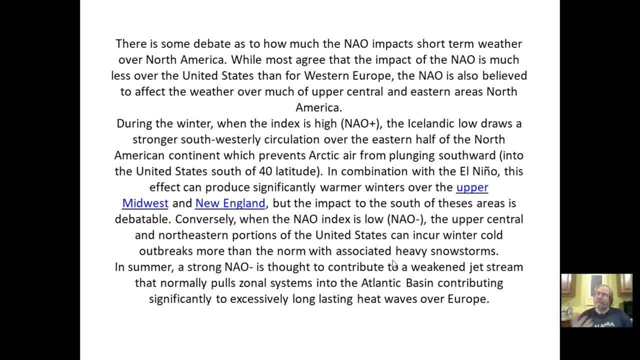 upper midwest and new england. now you notice being mentioned el nino here, mentioning arctic uh oscillation. right, that's what's implied here with the arctic air uh statement. all these systems are tied together. one big planetary difference between the arctic air and the southern half of the 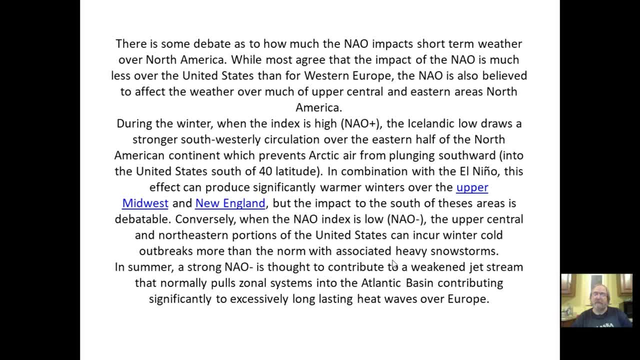 system. the impact of the southeast area is still uh being discussed and debated. when the nao index is low, negative, the upper central, northeast portions of the us can incur winter cold outbreaks more than the norm, with associated heavy snowstorms. because now what happens? the flow, instead of coming out of the southwest, coming out of the northeast, and what is new england known for. 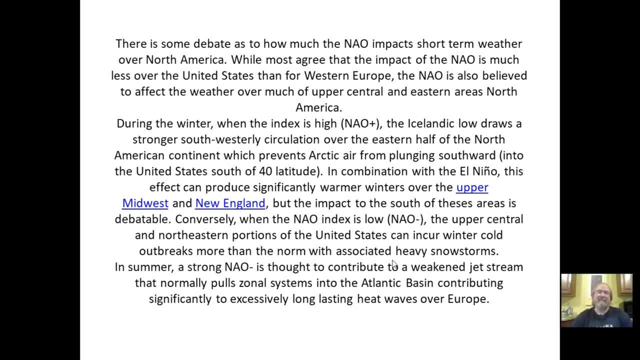 nor'easters, and some are strong negative. nao is thought to contribute to a weakened jet stream that normally pulls zonal systems into the atlantic basin, contributing significantly to excessively long-lasting heat waves over europe. now a brief word here. zonal systems are systems that flow in the basically east west west east direction. notice they follow latitudinal. 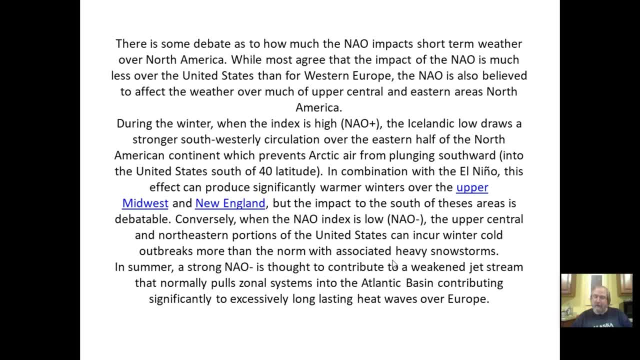 lines, then you'll hear: meridional systems, meridional systems are north, south, south north, following latitudinal- excuse me, longitudinal one. so zonal, follow latitudinal lines很好, follow longitudinal lines, okay. so when you see that, that's, that's what you need to remember under effects on the north. 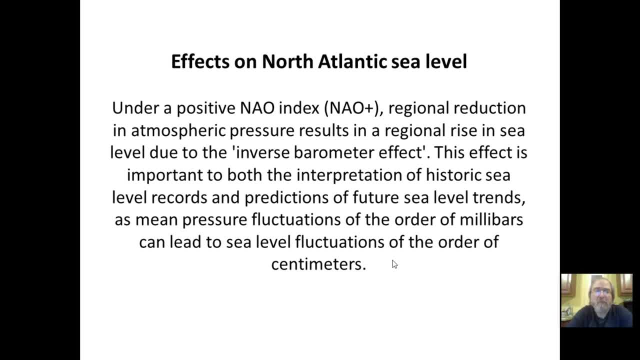 atlantic sea level. excuse me, under a positive nao index, a regional reduction in atmospheric pressure results in a regional rise in sea level due to the inverse barometer effect. If you're putting pressure over water and you reduce the pressure over the water, the water's gonna expand. 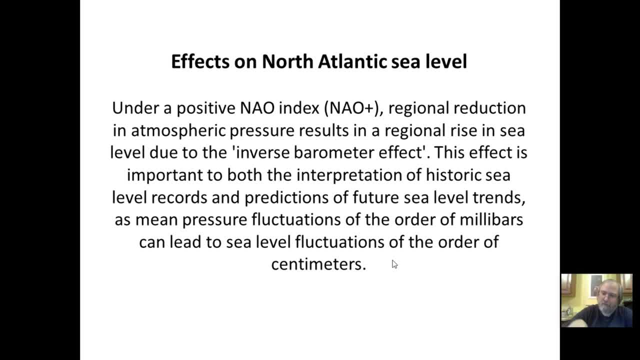 Putting high pressure on the water pushes the water down. We leave that pressure and the water's gonna expand. it's gonna rise up. This effect is important to both the interpretation of historic sea level record and predictions of future sea level trends, as mean pressure fluctuations of the order of millibars. 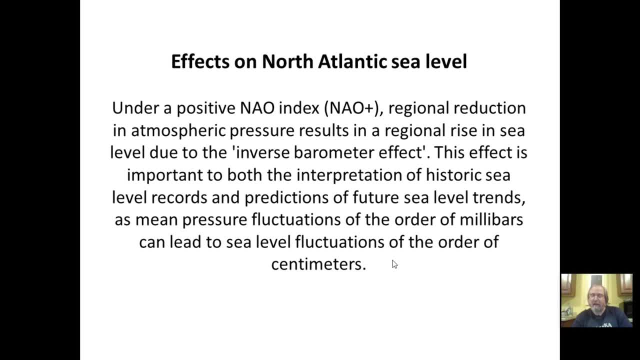 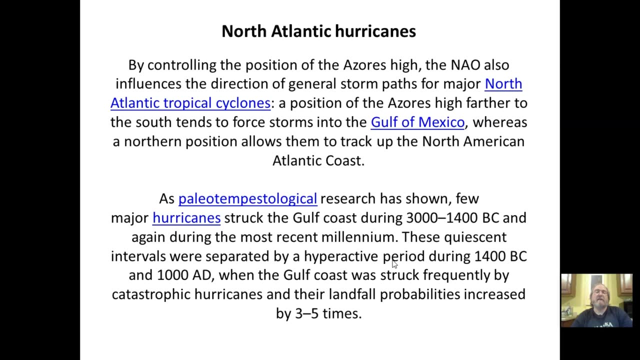 can lead to sea level fluctuations of the order of centimeters. And then you add in glacial melt from land ice and thermal expansion and you have those parameters to take into account. What about hurricanes in the North Atlantic Controlling the position of the Azores high? 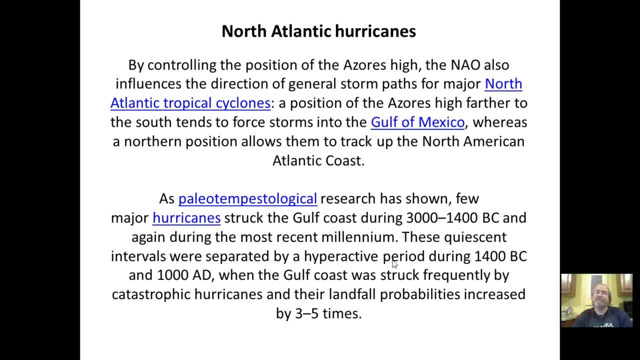 the NAO also influences the direction of general storm path for major North Atlantic tropical cyclones. low pressure system: A position of the Azores high farther to the south tends to force storms into the Gulf of Mexico Katrina, whereas a northern position allows them to track up. 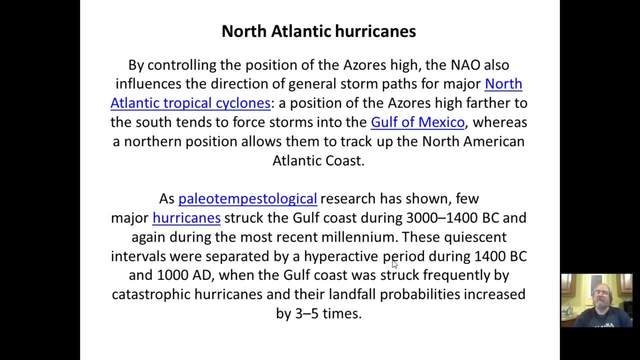 the North American Atlantic coast. So if you're in North Carolina, Virginia, watch out A paleotempestological research has shown tempestological tempest, storms and paleo. So this is, they say, looking at storms of the past. 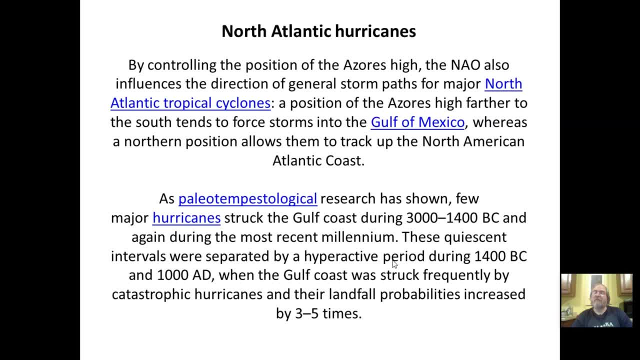 Few major hurricanes struck the Gulf Coast during 3,400 BC and again during the most recent millennium. These quiescent intervals were separated by hyperactive period during 1,400 BC and 1,000 AD, when the Gulf Coast was struck frequently. 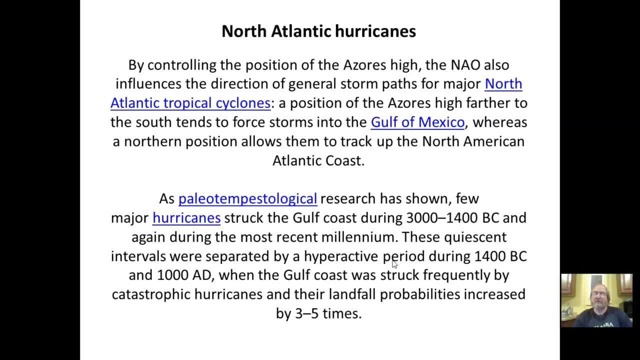 by catastrophic hurricane and the landfall probabilities increased by three to five times. So 3,000 to 1,400 BC. 3,000 to 1,400 BC. 3,000 to 1,400 BC BC. man not much slamming into the Gulf Coast. 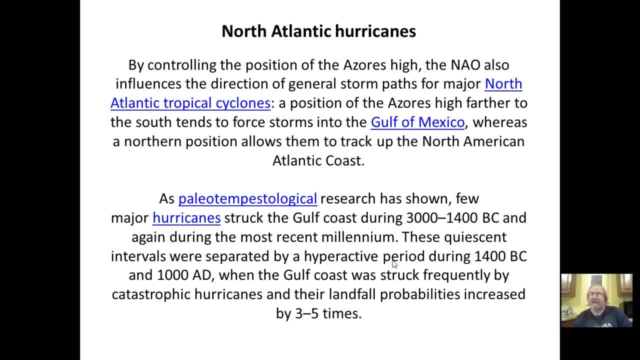 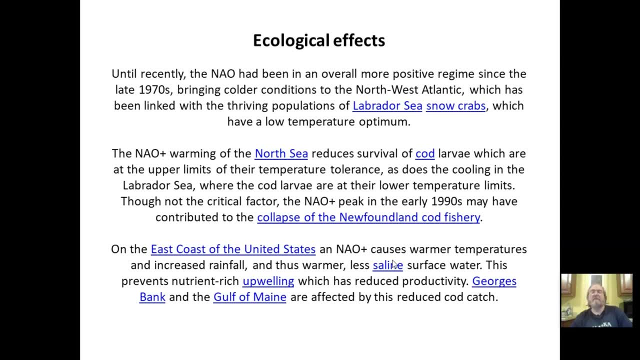 From 1,400 BC to 1,000 AD. it was getting the shit kicked out of it. basically is what they're saying. What about ecological effects? Until recently, the NANO had been in an overall more positive regime since the late 1970s. 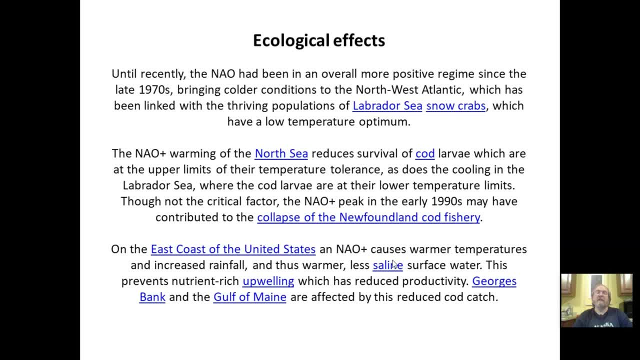 bringing colder conditions to the Northwest Atlantic, which has been linked with the thriving populations of Labrador sea snow crabs, which have a low temperature optimum. The NANO's positive warming of the North Sea reduces survival of cod larvae. they prefer cooler waters. 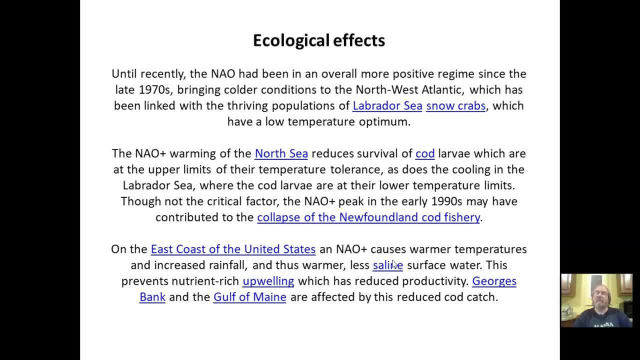 which are at the upper limits of their temperature tolerance, as does the cooling in the Labrador Sea, where the cod larvae are at the lower temperature limits, Though not the critical factor. the NANO positive peak in the early 1990s may have contributed to the collapse. 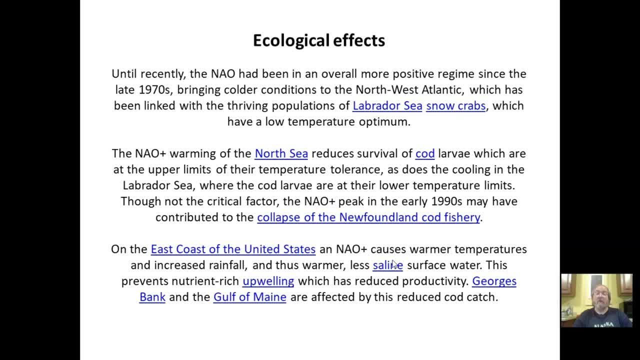 of the Newfoundland cod fisheries, along with overfishing. Let's not forget to add this: On the east coast of the US, a positive NANO causes warmer temperatures and increased rainfall. to thus warmer, less saline surface water. Less saline surface water means the water is not as dense. 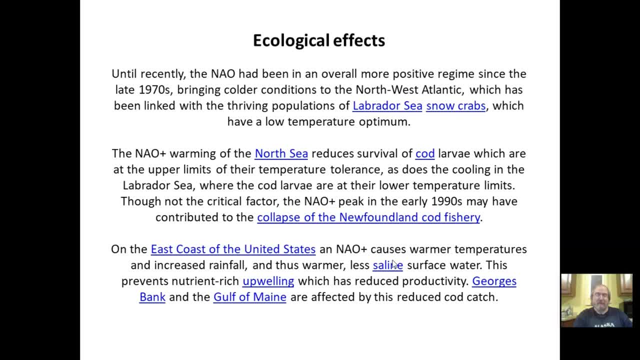 it's not going to sink This. this is important. this prevents nutrient-rich upwelling, which has reduced productivity because you're basically capping it off. The Georgia Spank and the Gulf of Maine are affected by this reduced cod catch. 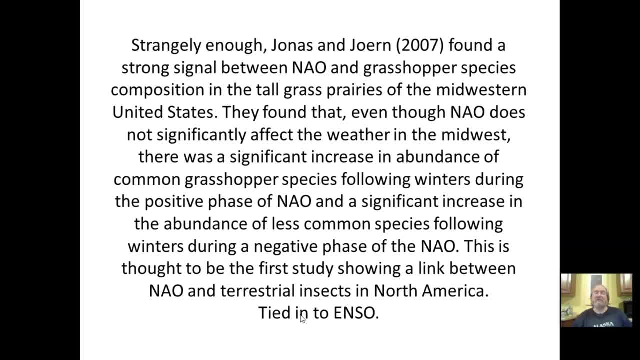 Now here's an interesting thing about. I just have to throw this in here. It doesn't show you how widespread the influences of these systems are. Jonas and Jern in 2007 found a strong signal between the NANO and grasshopper species composition. 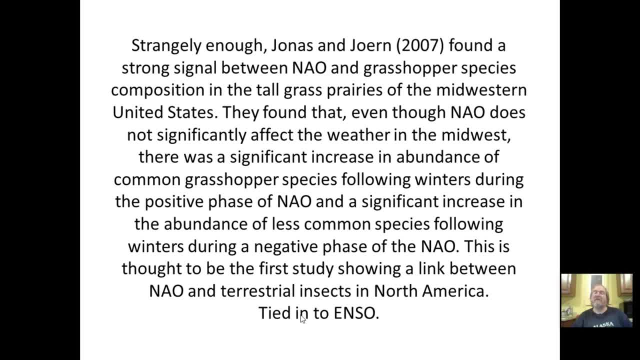 in the tall grass prairies of the Midwestern US. They found that, even though the NANO does not significantly affect the weather in the Midwest, there was a significant increase in abundance of common grasshopper species following winters during the positive phase of NANO. 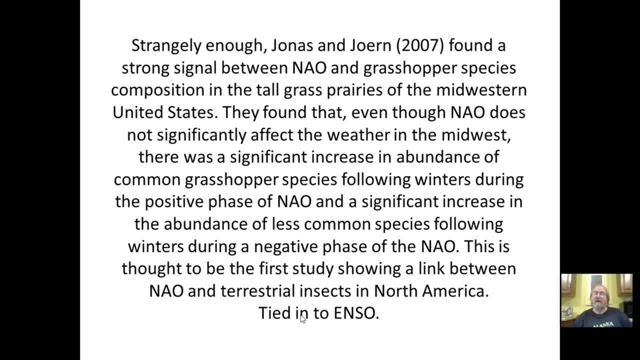 And a significant increase in the abundance of less common species following winters, during a negative phase of the NANO. This is thought to be the first study showing link between NANO and terrestrial insects in North America. And, by the way, you can now. 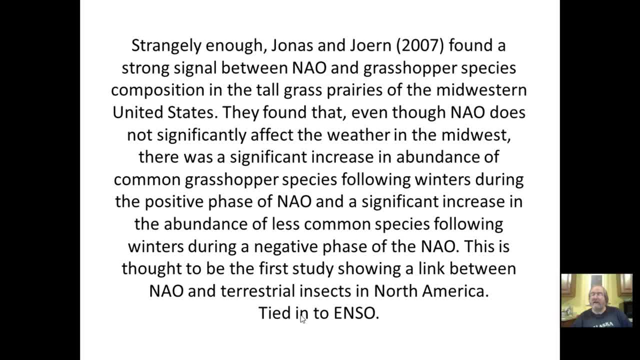 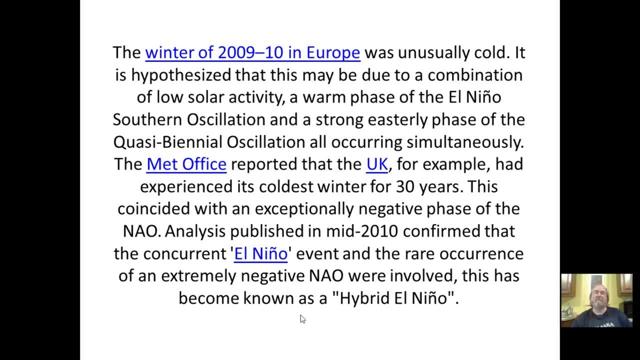 what goes on in North America. America is also tied into what happens with ENSO, as I showed you in that ENSO video. Now, the winter of 2009-2010 in Europe was unusually cold. It is hypothesized that this 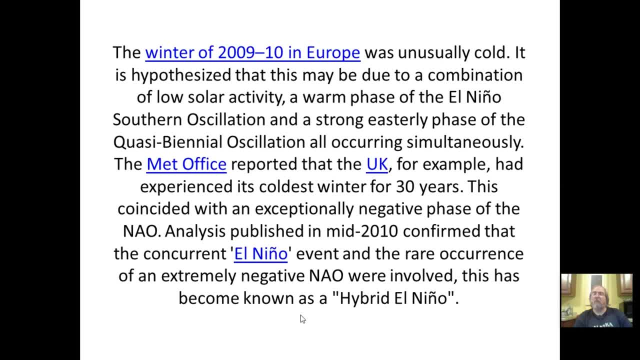 may be due to a combination of low solar activity, a warm phase of the ENSO and a strong easterly phase of the quasi-biannual oscillation, all occurring simultaneously. The Met Office, that's a major research group based in the UK, reported that the UK, for example, had experienced 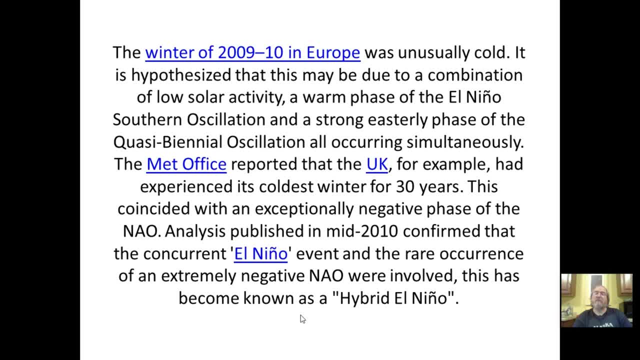 its coldest winter for 30 years. This coincided with an exceptionally negative phase of the NAO. Analysis published in mid-2010 confirmed that the concurrent El Nino event and the rare occurrence of an extremely negative NAO were involved, and this is now known as a hybrid El Nino. 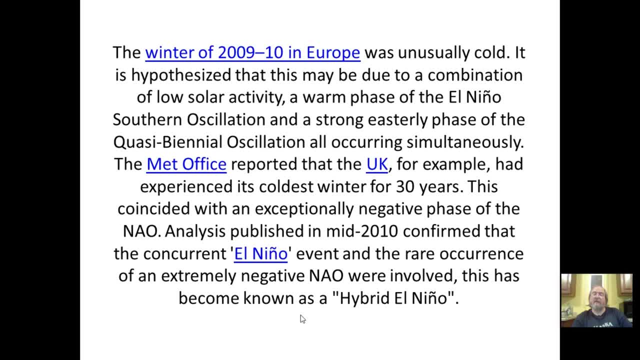 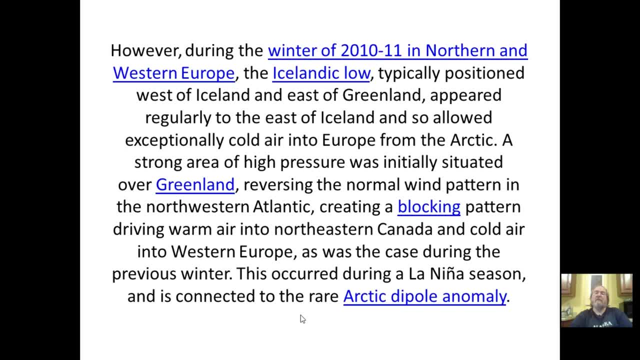 So a negative NAO with El Nino creates some pretty snotty conditions for Europe and the UK During the winter of 2010-2011. in northern Western Europe, the Icelandic low, typically positioned west of Iceland, east of Greenland, appeared regularly. 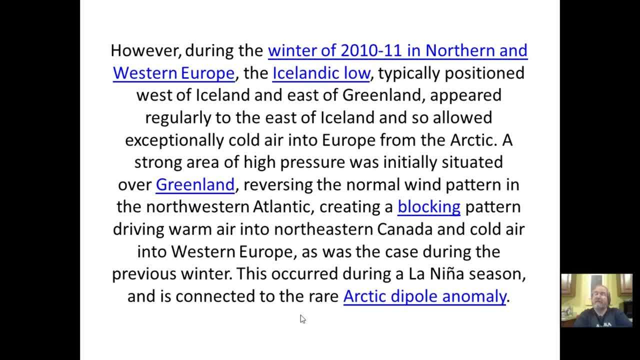 to the east of Greenland. The low, typically positioned west of Iceland, east of Greenland, appeared regularly to the east of Greenland, appeared regularly to the east of Greenland, appeared regularly to the east of Iceland. So it moved over significantly and so allowed. 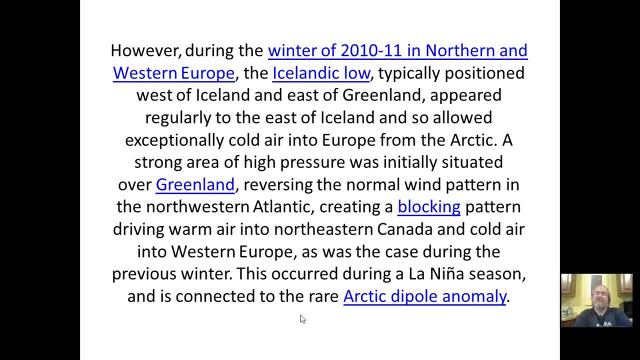 exceptionally cold air into Europe from the Arctic. A strong area of high pressure was initially situated over Greenland, reversing the normal wind pattern in the northwestern Atlantic, creating a blocking pattern driving warm air into northeastern Canada and cold air into western Europe. as was the case during the previous winter, This occurred during a La Nina season. 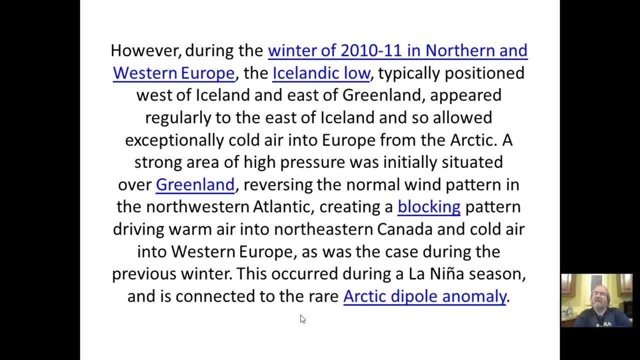 and it's connected to the Arctic Dipole Anomaly. I will have a video on the Arctic Dipole and spoiler alert. some people I used to work with at IARC, the International Arctic Research Center, were the ones that identified this, including a really excellent scientist, Dr John Walsh. 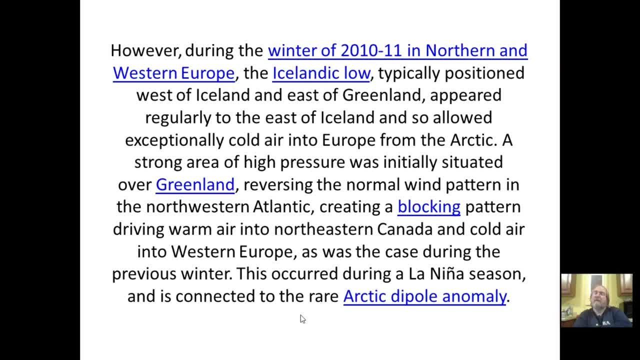 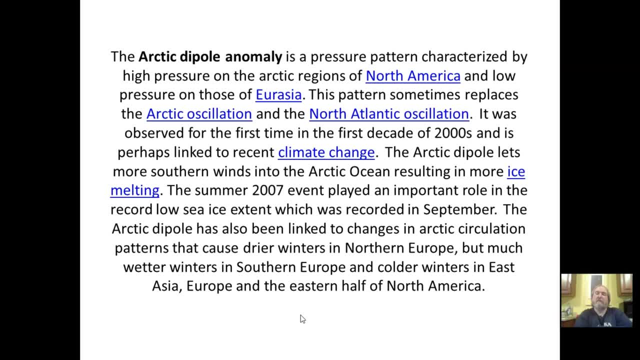 Great guy. Anyway, I will have a separate video on the Arctic Dipole That's coming up, And so I will just briefly mention here what this is. The Arctic Dipole Anomaly is a pressure pattern characterized by high pressure on the Arctic regions of North America. low pressure- 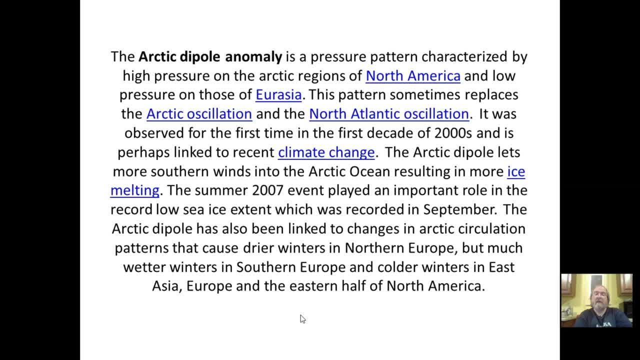 in those of Eurasia. This pattern sometimes replaces the Arctic Oscillation in the north Atlantic Oscillation. It was observed for the first time in the first decade of the 2000, and is perhaps linked to recent climate change. The Arctic Dipole lets more southern winds into the 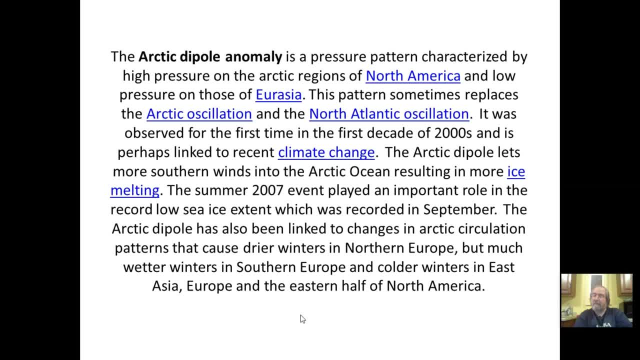 Arctic Ocean, and this is the Arctic Dipole, and the Arctic Dipole occupies much of the Arctic Ocean, resulting in more ice melting. The summer 2007 event played an important role in a record low sea ice extent, which was recorded in September. The Arctic Dipole- 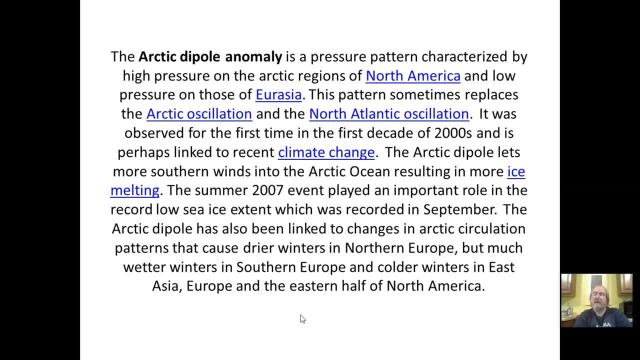 has also been linked to changes in Arctic circulation pattern that caused drier winters in northern Europe, much wetter winters in southern Europe, colder winters in East Asia, Europe and eastern half of North America. Depending on what the Arctic Dipole is doing, sometimes it will. in certain states it will keep the 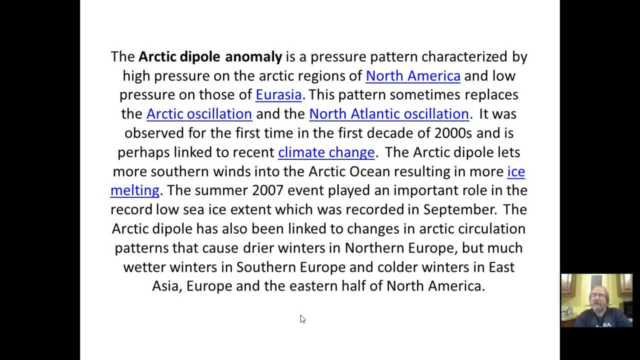 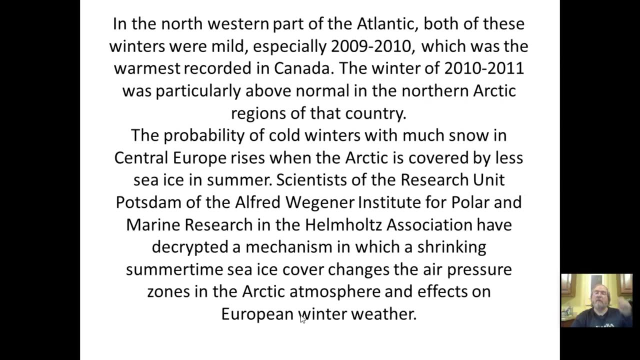 ice really contained tightly within the Arctic Ocean Basin. Other times it will increase the outflow of ice through the French Strait. That's it. I will be discussing that in a separate video soon. In the northwestern part of the Atlantic, both of these winters were mild, especially 09-10, which was the warmest. 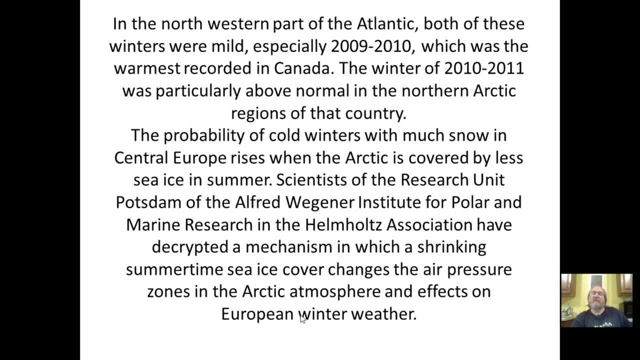 recorded in Canada, The winter of 2010-2011 was particularly above normal in the northern Arctic regions of that country. The probability of cold winters with much snow in Central Europe rises when the Arctic is covered by less sea ice in summer, because you can pull off more moisture from the water. Scientists 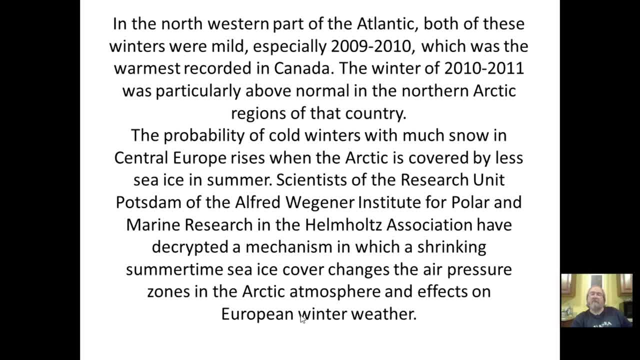 of the research unit Potsdam of the Alfred Wegener Institute for Polar Marine Research and the Helmholtz Association have decrypted a mechanism which a shrinking summertime sea ice cover changes the air pressure zones in the Arctic atmosphere and effects on European winter weather. Now there will be climate. 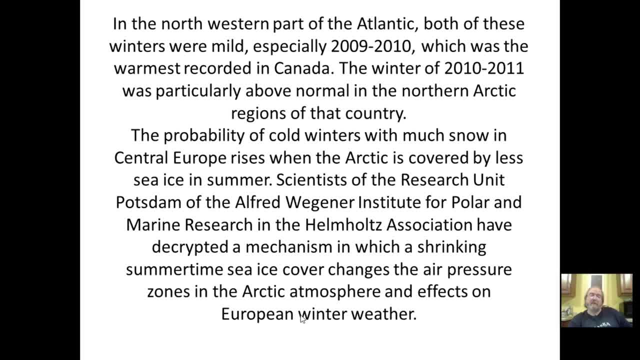 deniers of saying: see, this just shows, it's all variations and there's no such thing as global warming. Shrinking summertime sea ice cover is due to global warming. So what scientists do when they calculate the end of season? look at this. they look at. 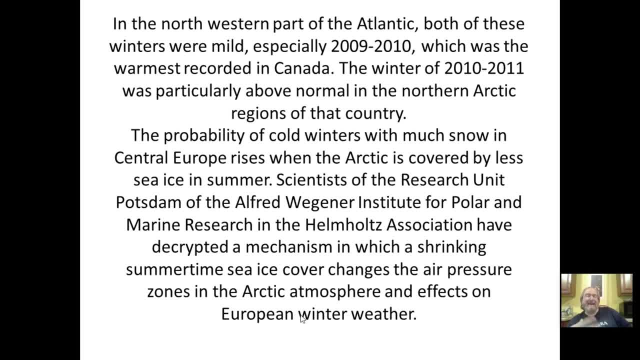 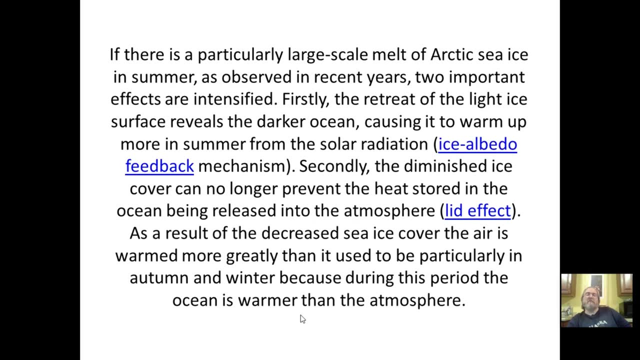 it, including the effects of global warming, and then they subtract out the effects of the global warming to calculate the indices to see what is happening. So they they look at it with and without It is accounted for. There's a particularly large scale melt of Arctic sea ice in summer, as observed in. 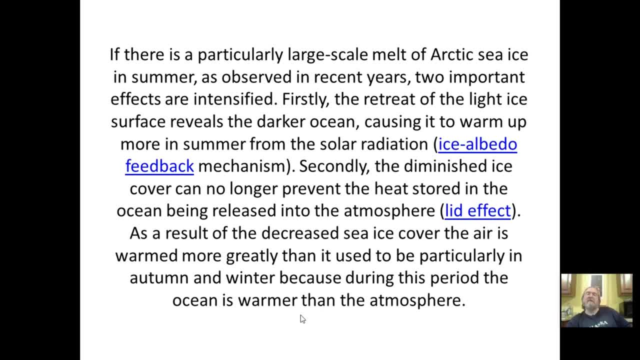 recent years. Gee, I wonder why Two important effects aren't intensified. Firstly, the retreat of the light ice surface reveals the darker ocean, causing it to warm up more in summer from solar radiation- The ice albedo feedback mechanism. In other words, if you have ice, the ice reflects the sun energy. 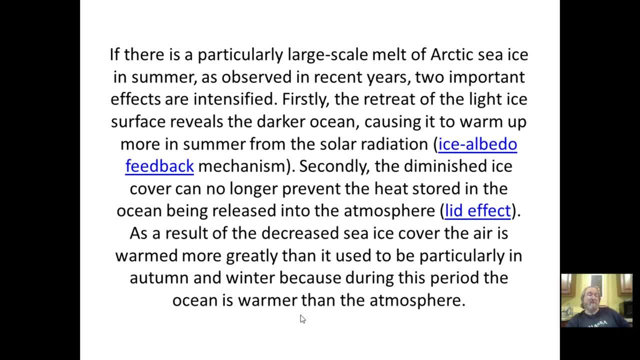 back into space. No ice, you have water. the water absorbs. Ice cover can no longer prevent the heat stored into the ocean being released into the atmosphere. It's called the LID effect. In other words, whatever heat's in the water, if there's. 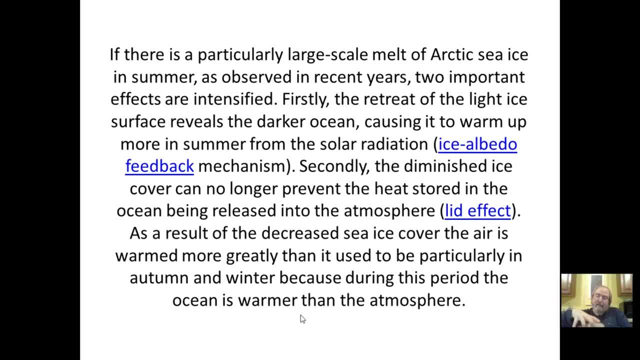 ice over it. the ice is a cap. it prevents that heat from being released into the atmosphere. no, no arctic sea ice. nothing preventing that heat from going right into the atmosphere. that's basically what's happening. as a result of the decreased sea ice cover, the air is warm more. 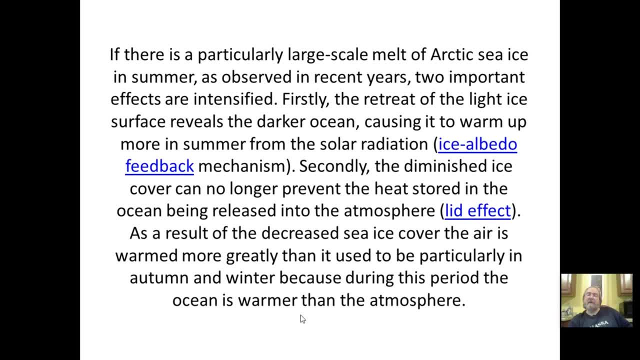 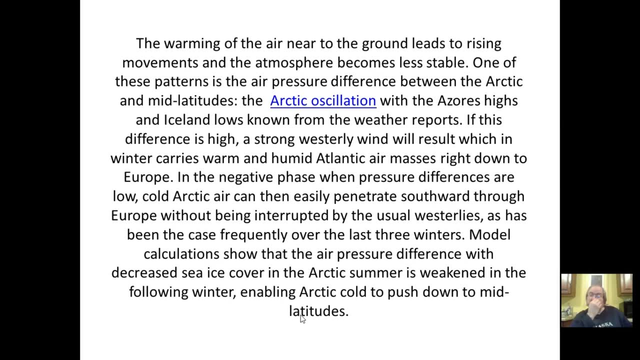 greatly than it used to be, particularly in autumn and winter, because during this period the ocean is warmer than the atmosphere. you know the reason why alaska has been having nice, mild winters lately: the warming of the air near to the ground leads to rising movements. right, we discussed that with 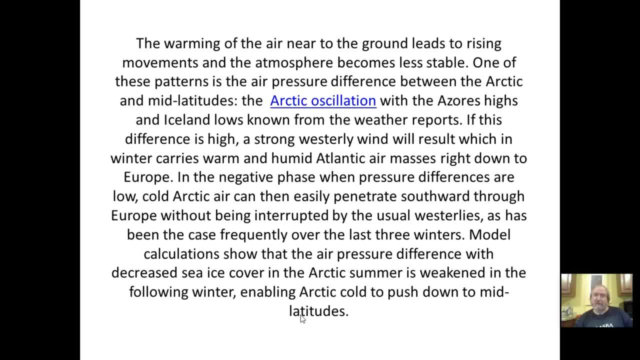 low pressure system and the atmosphere becomes less stable. we discussed that low pressure system. one of these patterns is the air pressure difference between the arctic and mid latitudes, the arctic oscillation with the azor high and iceland lows known from the weather reports. if this difference is high, 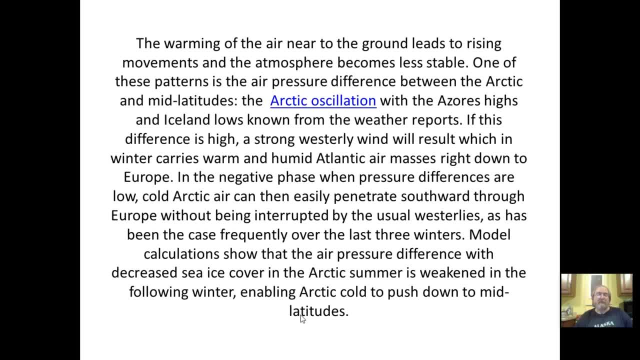 pressure gradient right. i discussed that in the rotating system video. if this difference is high, a strong westerly wind will result, which in winter carries warm, humid atlantic air masses right down to europe, usually during the positive phase. in the negative phase, when pressure differences are low, not as great, cold arctic air can then easily penetrate southward through europe. 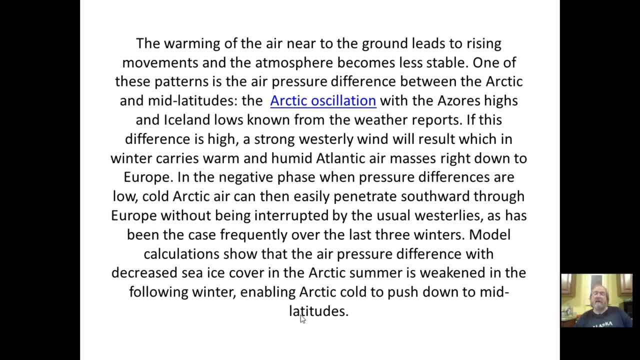 without being interrupted by the usual west always has been the case, frequently over the last three winters. model calculations show the air pressure difference: with the decreased sea ice covering the arctic summer is weakened in the following winter, enabling arctic cold push down to mid-latitude. oftentimes this is accompanied by the jet stream dipping down, and we'll see that later on. 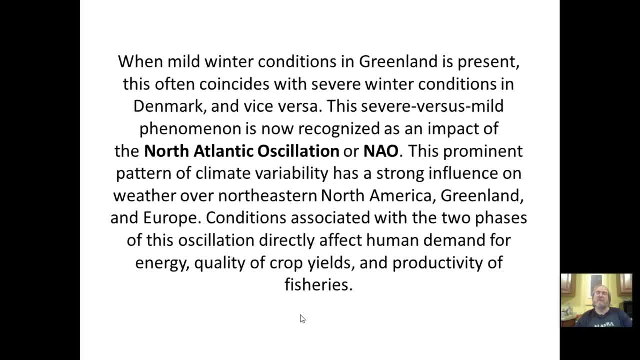 when mild winter conditions in greenland is present, this often coincides with severe winter and vice versa. This severe versus mild phenomenon is now recognized as an impact of the NAO. This prominent pattern of climate variability has a strong influence on weather over Northeastern North America, Greenland and Europe. 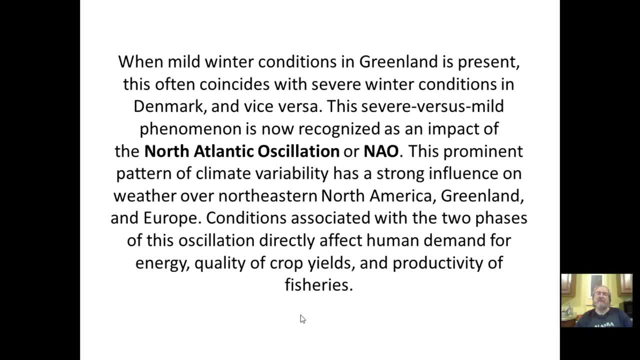 Conditions associated with the two phases of this oscillation directly affect human demand for energy, quality of crop yield and the productivity of fisheries, And this is all being affected by global warming. Do not kid yourselves about that. It is happening. This is a changing, this global warming. 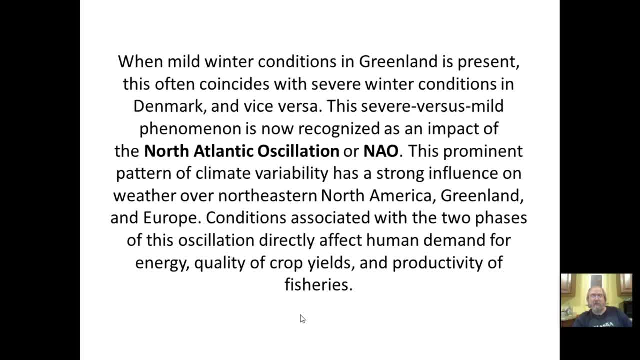 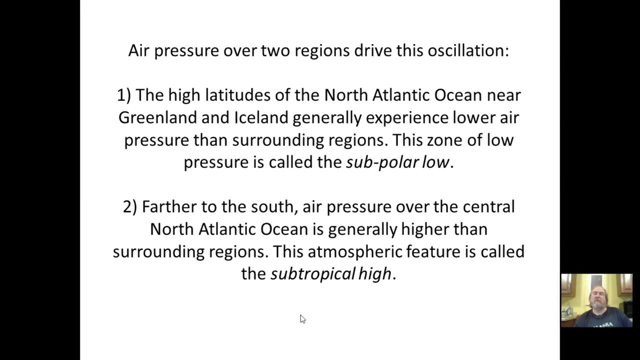 is changing how these systems, and so IPO, PDO, NAO, AO, AMO, whatever, all affecting how these systems are behaving. Air pressure over the two regions drives this oscillation. The high latitudes of the North Atlantic Ocean, the Greenland. 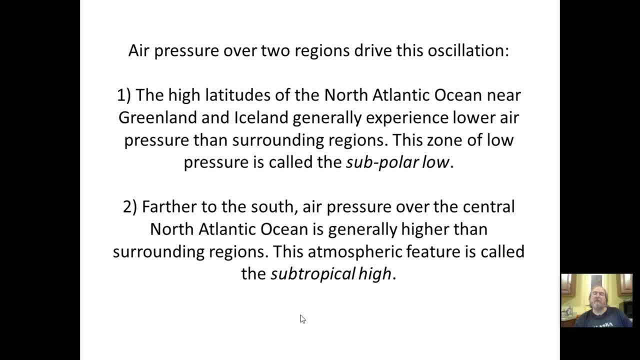 and IAEA Iceland generally experienced lower air pressure than surrounding regions. This zone of low pressure is called the subpolar low. I showed that to you in the rotating systems video. Farther to the South, air pressure over Central North Atlantic Ocean is generally higher than surrounding regions. This atmospheric 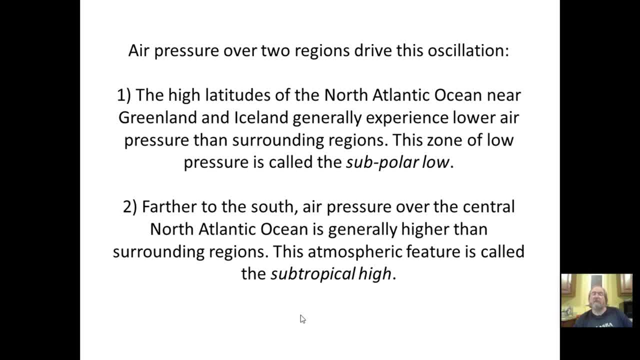 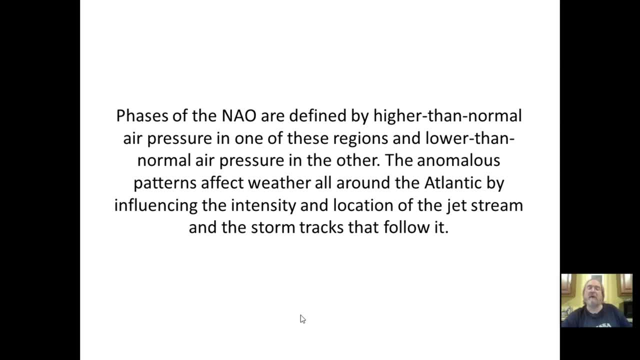 feature is called the subtropical high. Again, I showed that to you in the rotating systems video. Phases of the NAO are defined by higher atmospheric pressure than the surrounding regions: High atmospheric, higher than normal air pressure in one of these regions and lower than normal. 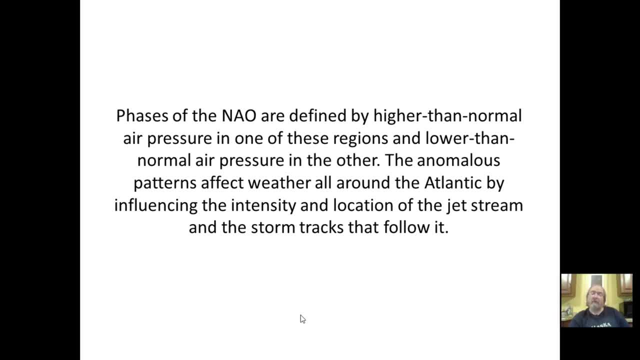 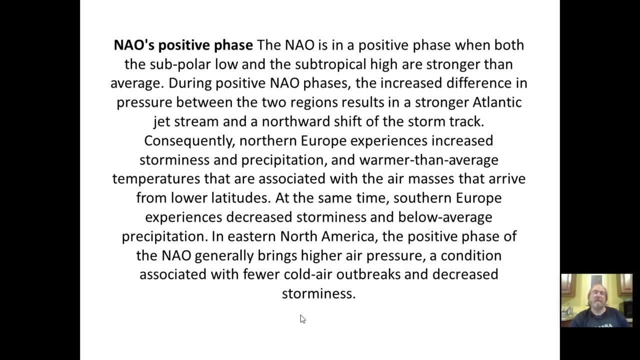 air pressure in the other and they flip-flop back and forth, They oscillate, hence the NAO acronym. The anomalous patterns affect weather all around the Atlantic by influencing the intensity and location of the jet stream and the storm tracks that follow it. The NAO's positive phase. It's in a positive phase. 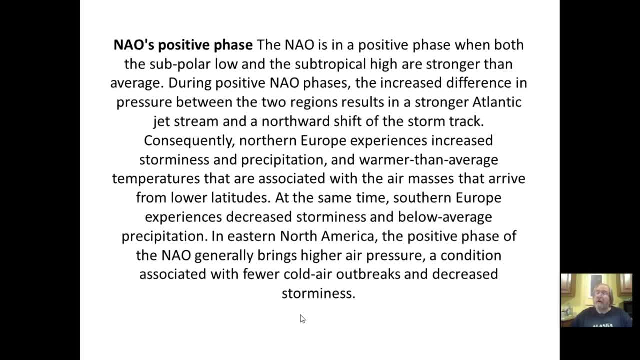 when both the subpolar low and the subtropical high are stronger than average During positive NAO phases. the increased difference in pressure between the two regions result in a stronger Atlantic jet stream and a northward shift of the storm track. Consequently, Northern Europe experiences increased 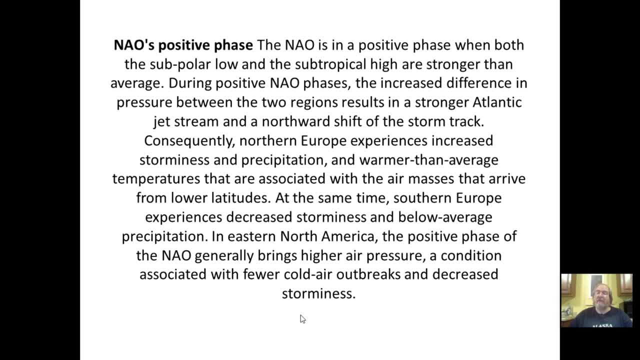 storminess and precipitation and warmer than average temperatures that are associated with the air masses that arrive from lower latitudes. At the same time, Southern Europe experiences decreased storminess and below average precipitation. In Eastern North America, the positive phase of the NAO generally brings higher air pressure, a condition. 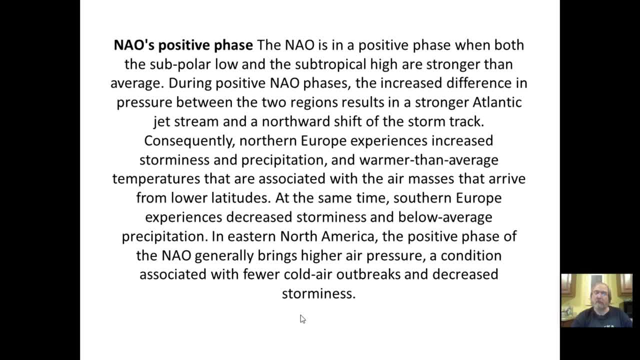 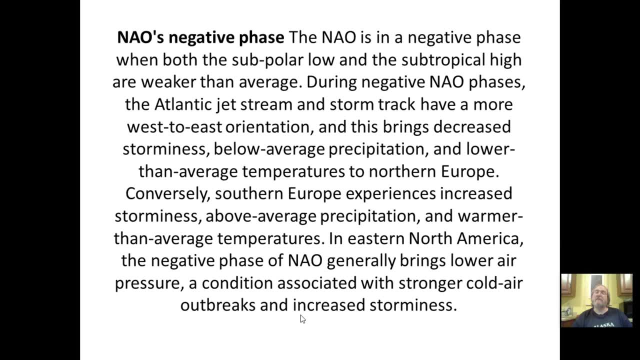 associated with fewer cold air outbreaks and decreased storminess. Guess what happens during the negative phase? It's in a negative phase when both the subpolar low and the subtropical high are weaker than average. During negative NAO phases, the Atlantic jet stream and storm track have a more west-to-east. 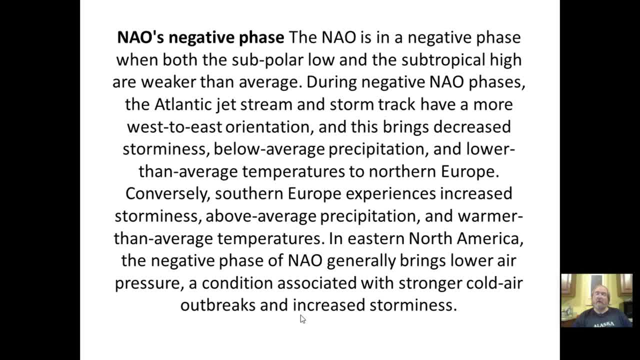 orientation, and this brings increased storminess, below average precipitation, lower than average temperatures to Northern Europe. Conversely, Southern Europe experiences increased storminess, above average precipitation, warmer than average temperatures. In Eastern North America, the negative phase of NAO generally brings lower air pressure, a condition associated with stronger cold air. 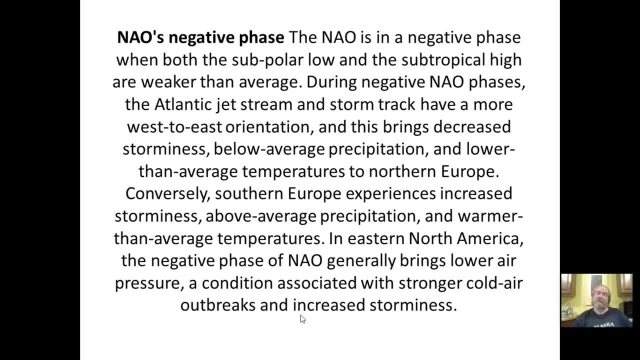 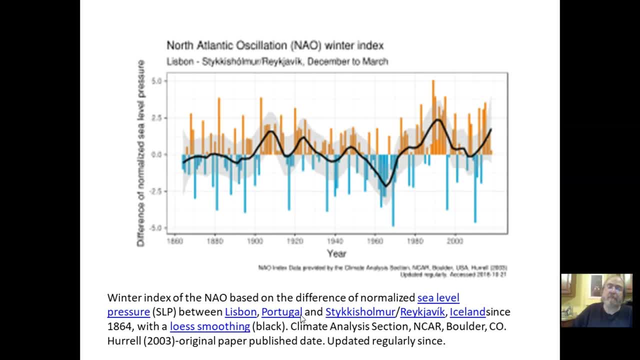 outbreaks, increased storminess, including the famous nor'easters of New England. Now we get to some examples for all these measures to help us understand the effects of the impact on the Arctic Coast. What you see here are two more of the major. uh yeah, about the 2017 or so. so this is the winch of the index of the nao, based on the difference. 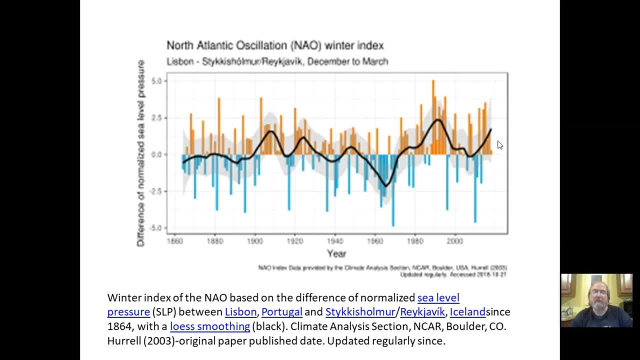 of normalized sea level pressure. now that refers to hemisphere pressure at sea level, not sea level height, between lisbon, portugal, and, uh, the stuka sholmur rickovich, iceland, since uh, 1864, with a lurce smoothing. that's this black line here, showing some sort of a oscillatory pattern. 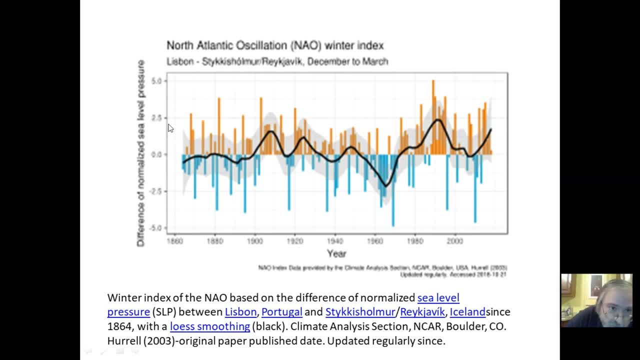 and if you look at the scale here, okay, the blue is the negative phase and i guess call this brown, that's the positive phase. so this is nao positive, this is nao negative. this is the difference of the normalized sea level pressure, what we just discussed in the previous two slides, the 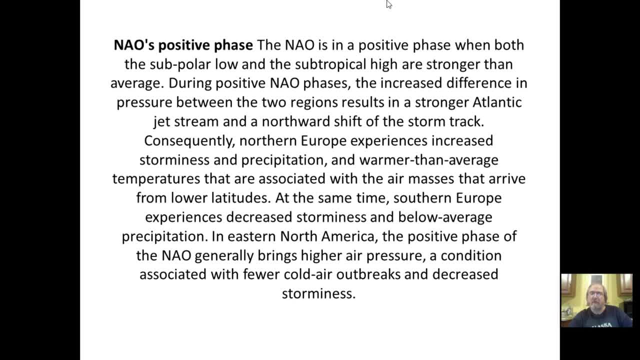 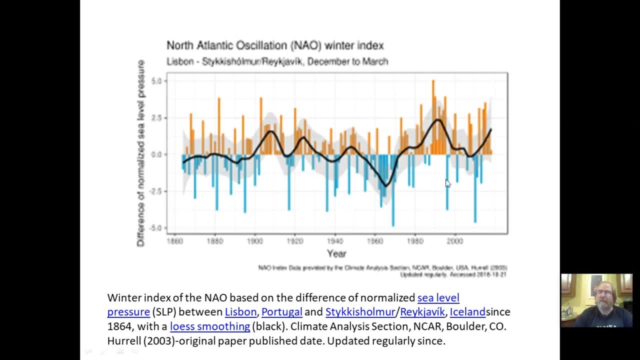 the relative strength of the sub subpolar and subtropical highs. and this is uh from ncar, national center for atmospheric research in boulder, colorado. uh, the original paper is herald 2003, but it keeps being updated regularly. so 2003 is here and it just keeps being. 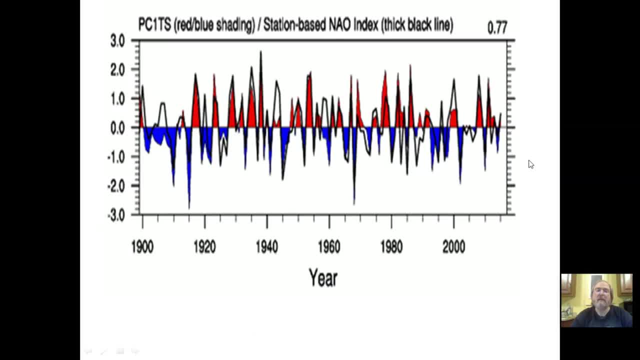 updated, so continued work. okay, so this is the uh nao looking narrowing down the range from 1900 to basically it looks like about 2016 or so. so this is uh. the thick black line is the station based nao index and then the red blue shading is this other group. 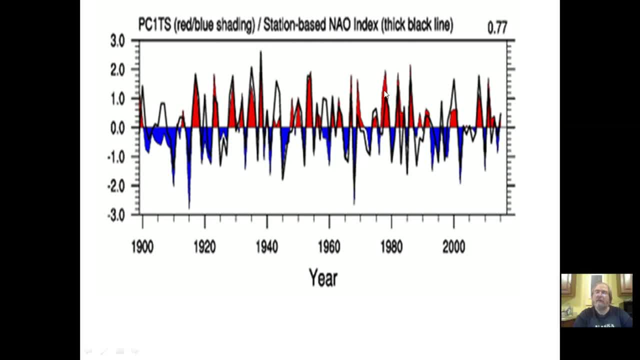 doing that. but basically, again, you can see how it flips back and forth- is what this is showing. okay, um, some really uh, this is probably a very strong negative phase here, so it probably has some really nasty conditions in the eastern us, eastern north america and you know likewise some very strong positive naos. 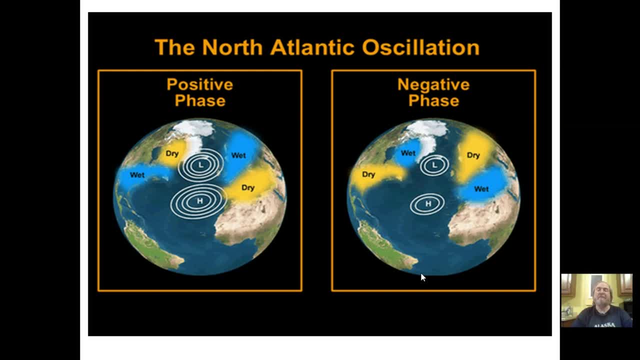 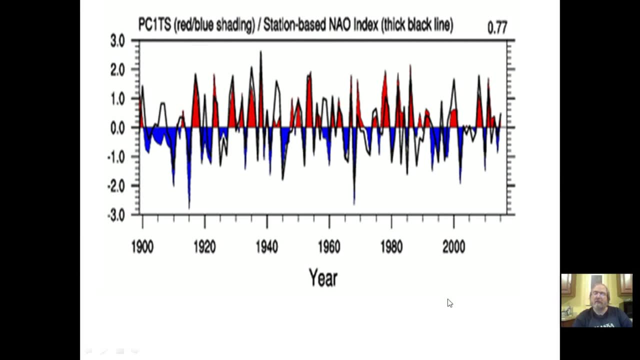 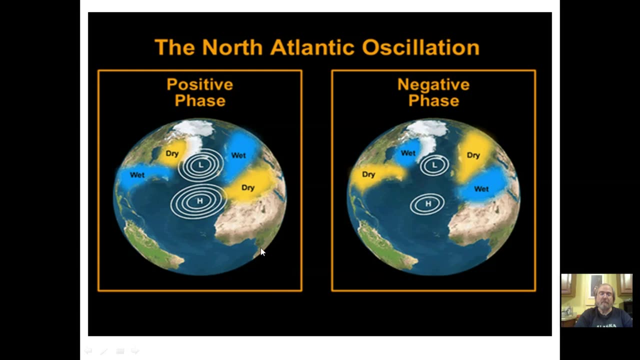 there as well. okay, i like this uh diagram, so i like showing indices because they in this you can see at quick glance the oscillatory nature over time. this is showing what's going on here. so here's the icelandic low, here's the azores high. 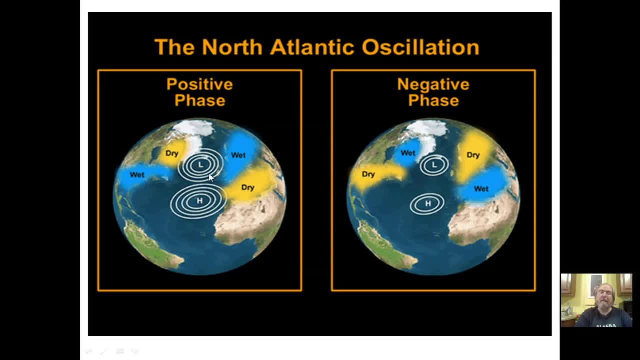 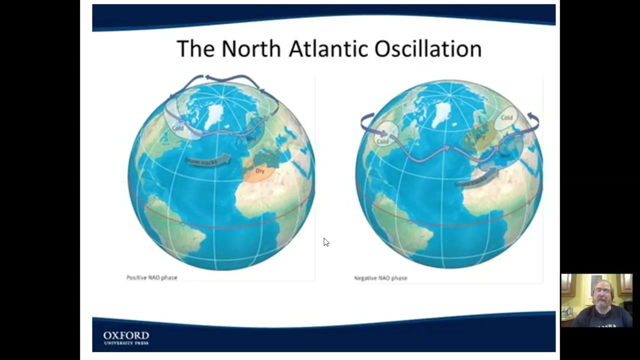 right. more contour lines mean they are stronger. okay, they're weaker here. so we have wet conditions and dry conditions. wet conditions, dry conditions. you see how they flip-flop: on the positive phase to the negative phase. they flip-flop. okay, now this is what it does to the flow of the jet stream. right, so on the 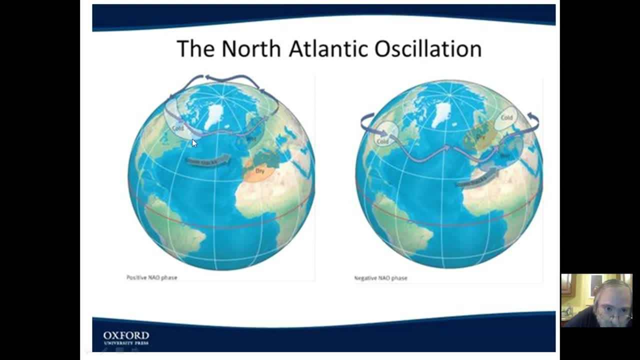 left. here is the positive phase. okay, cold air being here. you can see it is a. it is constrained to a more northerly track. this is going to be wet and dry right. wet and dry right, showing that, and it's very, very tight. no gesturing. 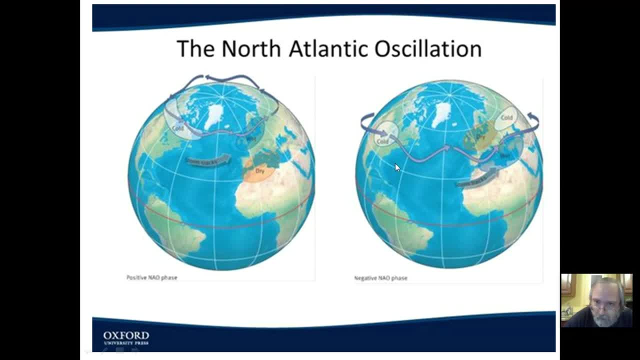 close to uh, to polar regions. in the negative phase it meanders and dips down further south. now we get cold conditions here, wet conditions, and so it's going to be a little bit different than what we saw in the southern europe, in the mediterranean region. 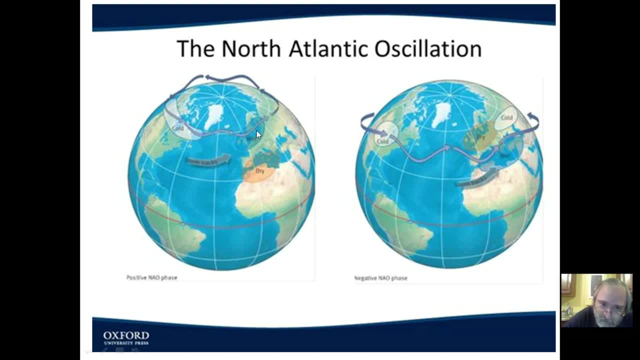 dry conditions over southern scandinavia, northern europe- right, it's wet over scandinavia and northern europe- dry over southern europe and the mediterranean. the cold is kind of like basically at the us- canadian border here, but it drops down because the storm track brings it down into the midwest. so positive, negative phase of the north. 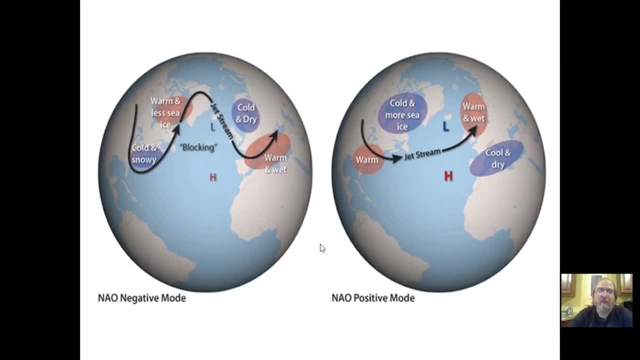 atlantic oscillation and this is just. uh, we i mentioned earlier the blocking. this is what's meant by the blocking, where you know it prevents the pressure systems from moving around. as you can see, it dips down low, very cold, snowy condition to south eastern north america: warm and less sea ice. 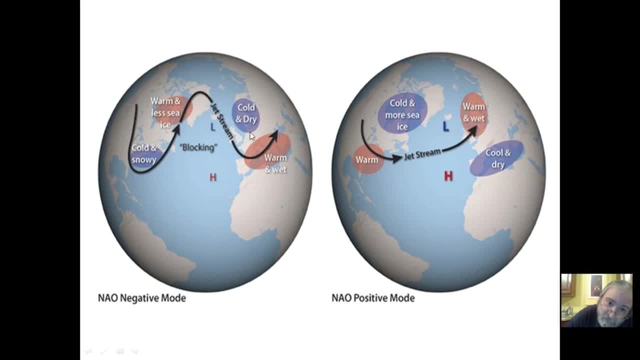 cold and dry over scandinavia, parts of northern europe. warm and wet over southern europe and the uh mediterranean. you've got a weak and high and a weak and low and it kind of and it blocks, so the jet stream moves up and over. that's in the negative mode. the positive mode, you see the jet. 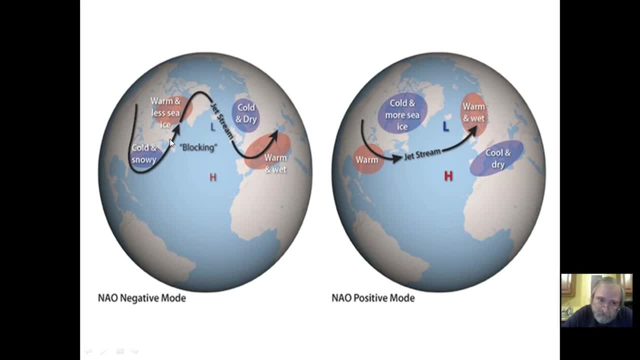 stream is more direct, more zonal flow, it's just kind of meridional. it's more nerdy on dipping down and it's more it's more of a westerly track like west to east. now you have cold, more sea ice. it's warm, warm and wet. 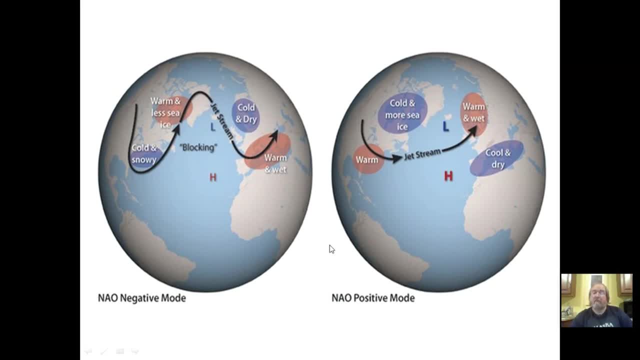 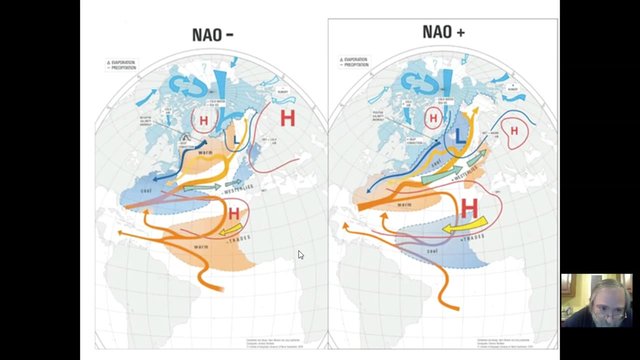 cold and dry. again, it flip-flops. it literally does oscillate. notice the the pressure system strength, and this is just showing some really fun tracking stuff here. um, you know, it gives you a little more detail: high pressure, low pressure here. so, um, here's the high off the azores. this is the low of. 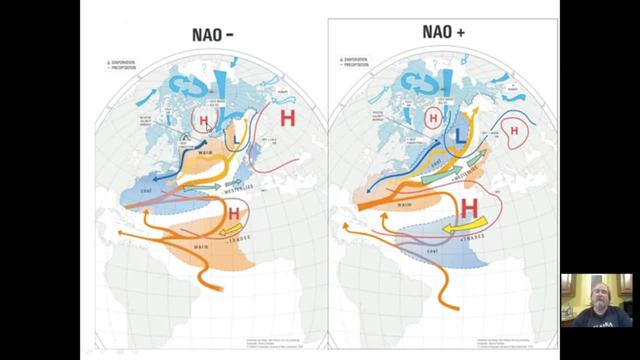 the icelandic low and remember how showed you in the rotating systems video that the high pressure system and low pressure system often occur next to each other because of the- remember the air pressure is moving in 3d and so where you have a convergence in the low, 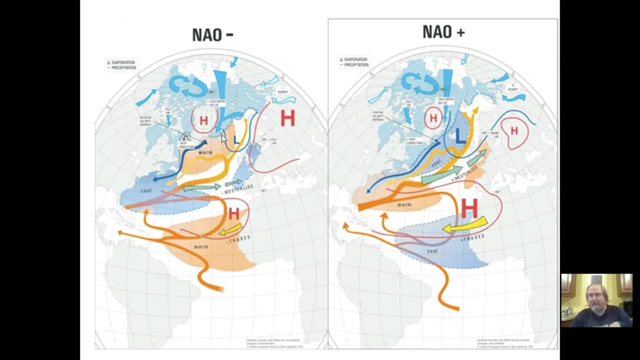 pressure system at the base and divergence at the top. that leads to a convert: convergence at the high, pressure at the top and the divergence at the bottom. you create those vertical convection cells. positive phase: the days or high strengthens, as does the Icelandic well, and you can see what. 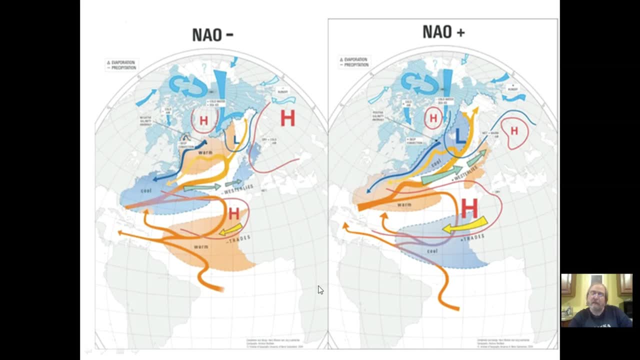 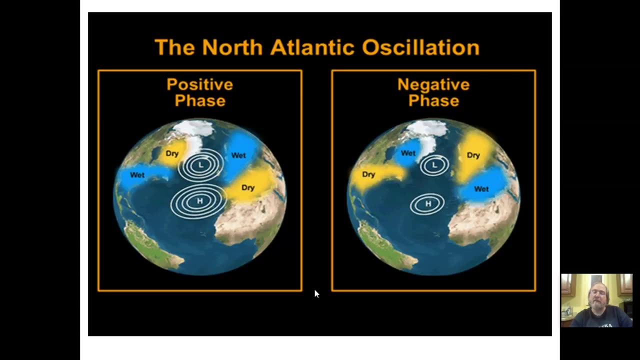 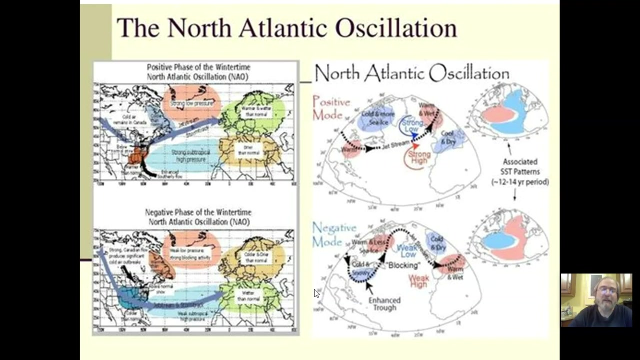 happens with the storm tracks. we can, you can look at this a little closer detail. pause the video, stare at it for a bit, but that these, these series of videos, kind of tell you story what's happening, and then this gets even more fun, trying to show you how everything is just intertied together. so the positive 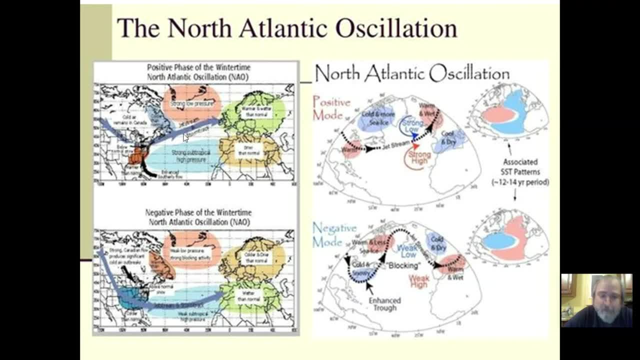 phenomenon of ascendancy. this again, we probably know that for tensile energy, events are hard and some of you have these things that are ways ofhibition or something like that. so if you're a consumer now, you might want to take a phase of the wintertime North Atlantic Oscillation. 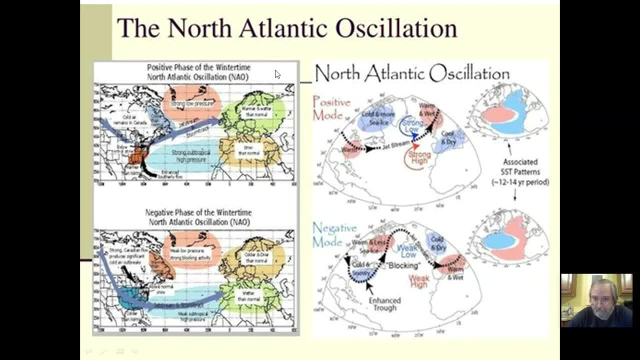 And a lot of attention is paid to the wintertime because of the severity of the winter that people in various locations will experience. And so you have the strong low pressure here, strong subtropical high pressure. here the jet stream brings it in. 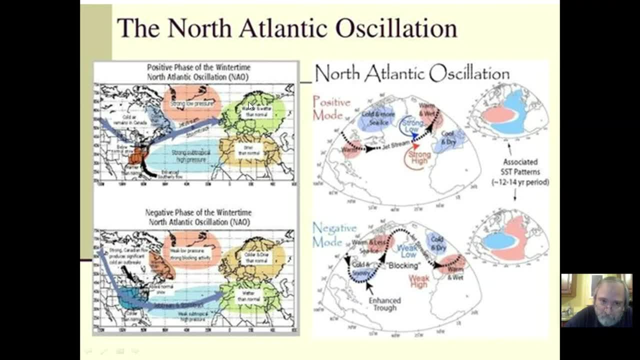 you get warm weather than usual in Northern Europe, Scandinavia, drier than usual over Southern Europe and Mediterranean, And again cold, more sea ice, stronger, low, stronger high, warm and wet. It just brings the storm bang right over it, right. 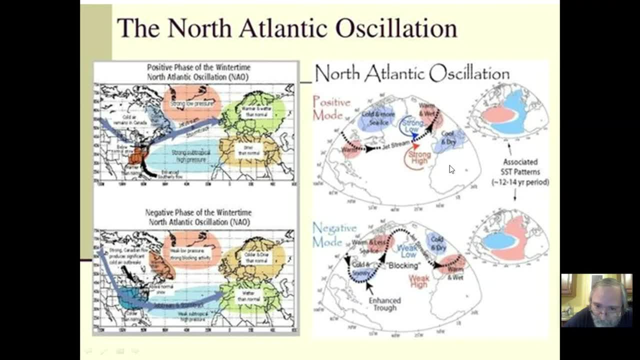 Brings it right over the top- cool and dry- here, Whereas in the negative mode the blocking prevents that storm trap from slamming- that you know slamming- warm, wet weather over Northern Europe and Scandinavia. It dips down, leaving them cold and dry. 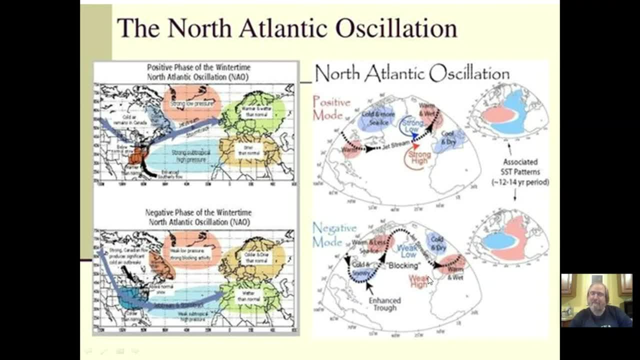 And then Southern Europe gets hit with the wet stuff And you can see what's happening here. The storm track goes further south. So, as always, you can feel you know in viewing these videos. you know, pause the video and examine these slides here. 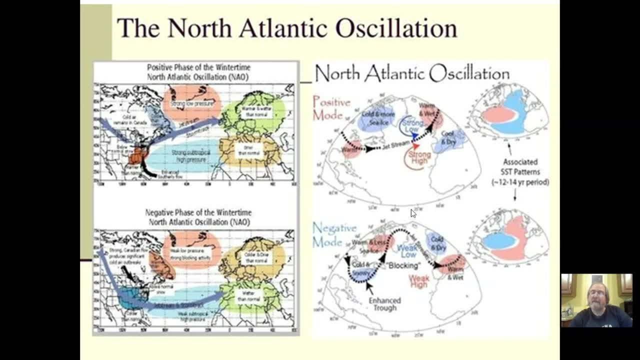 There's a lot of information. SST, of course, is sea surface temperature. I'm not going to really discuss that too much. Instead, the NEO looks more at the air pressure. You know, of course. you know, depending on the storm track there. yeah, 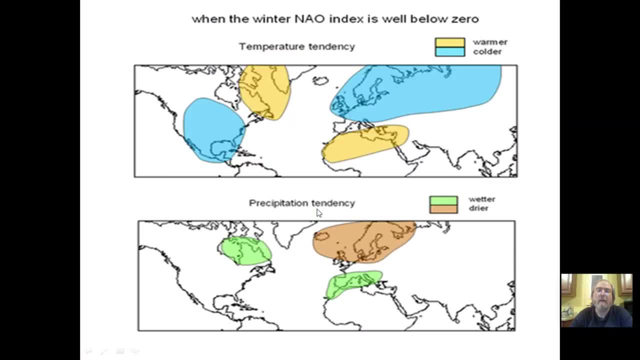 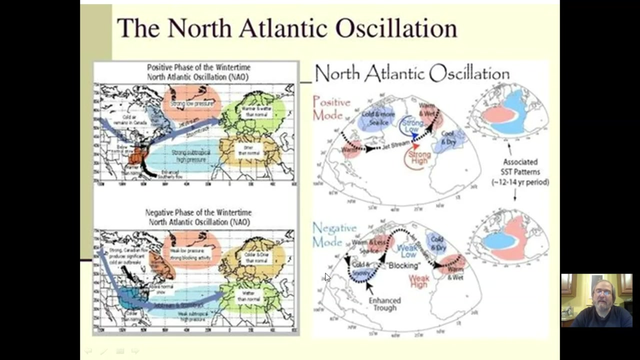 you know it's going to affect the sea surface temperature somewhat When the winter NEO index is well below zero. in other words, negative mode. That tan is warmer, blue is colder, precipitation wetter and drier. right and it's drier, that's wetter, it's kind of. 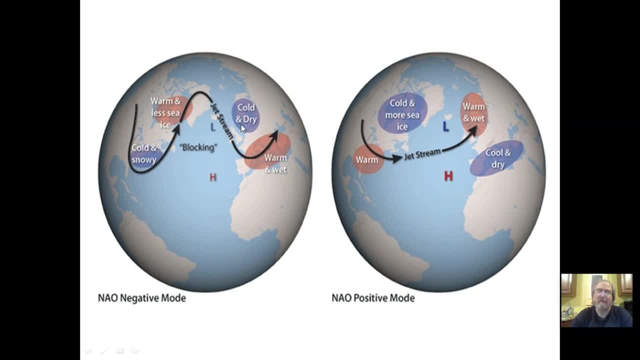 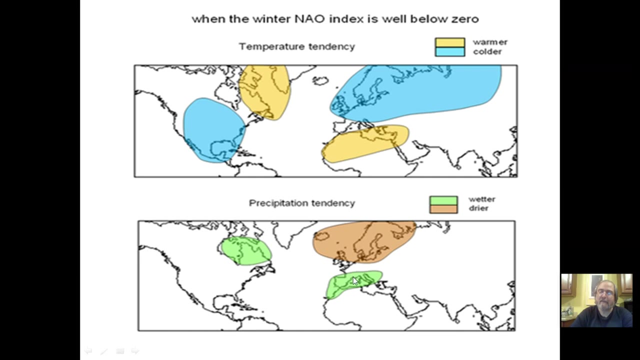 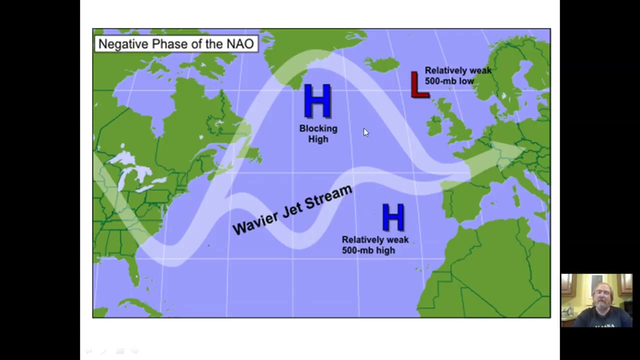 you know that's the positive. negative away, so wetter, drier, cold and dry for the negative mode. and wet down there, so cold and dry, warm and wet, cold and dry. there we go. so this is showing the world below zero. this is in the negative phase, negative phase of the NAO. you get the wave here, the blocking high, you get. 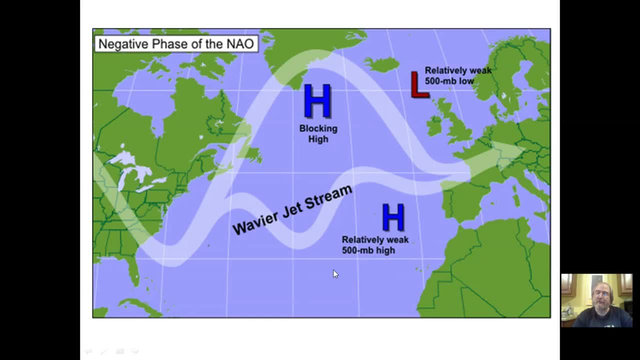 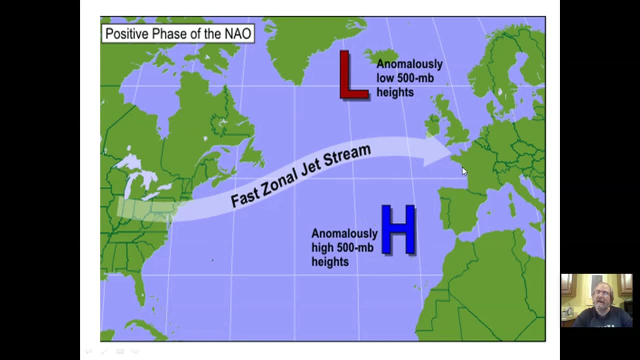 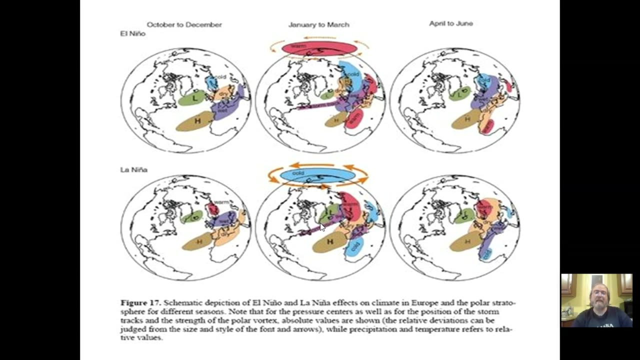 the wave, your jet spring, versus the positive phase with fast zonal right following, latitude in the lines. just bang right in there, okay. so what I want to do i wanted to show you know- El Nino and the top here and La Nina down here- and what I wanted to do to show how it kind of ties in with 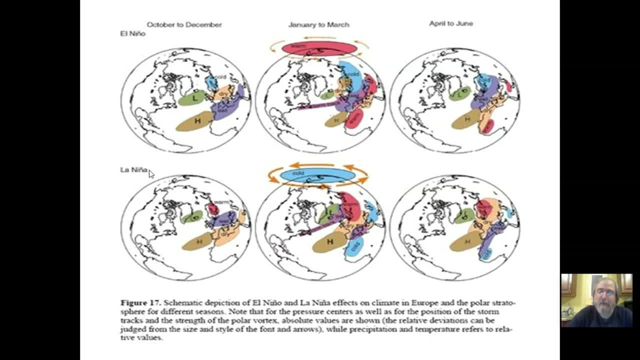 what's going on with the NAO. so here's a El Nino. we have an El Nino April, December, January to March, April to June. so what's missing is July, October, the september, basically those three months. but what we see here is okay. it is the low there's. 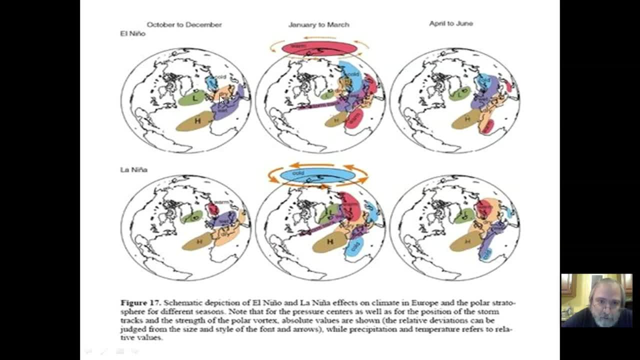 the high there's, you know, cold, dry, so we know that's going to be. uh, that's, that's what's happening in the lino and la nina. here's the positive track here. right, this is the winter months. here is the positive track. this is the nao and the positive here: cold air at the top here. so 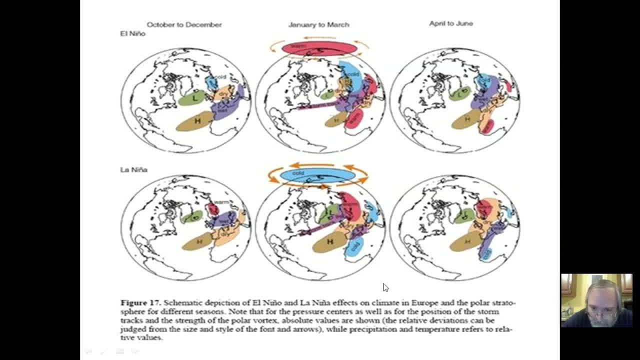 the schematic showing the depiction of el nino, la nina, effects on climate in europe and the polar stratosphere for different uh seasons. that's come on. that's this here. polar stratosphere. note that for the pressure center, as well as for the position of the storm track and strength of 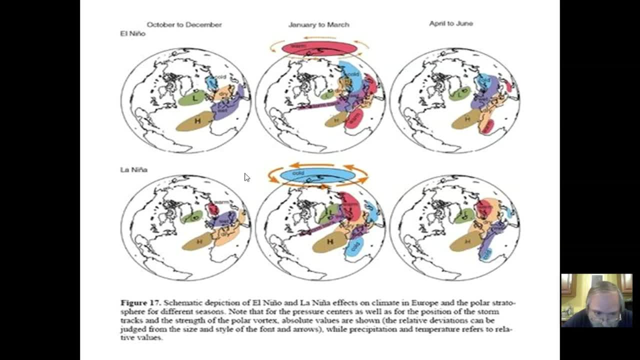 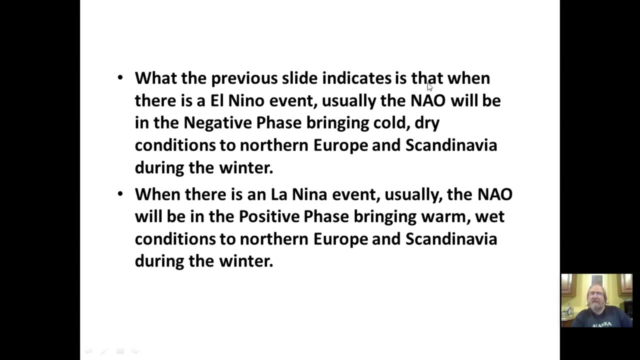 the polar vortex, absolute values are shown. relative deviations can be judged for the size and style of the font and the arrows. okay, precipitation and temperature refers to relative values. okay, what the previous slide indicates is that when there is an el nino event, the nao typically will be in the negative phase, bringing cold, dry conditions. 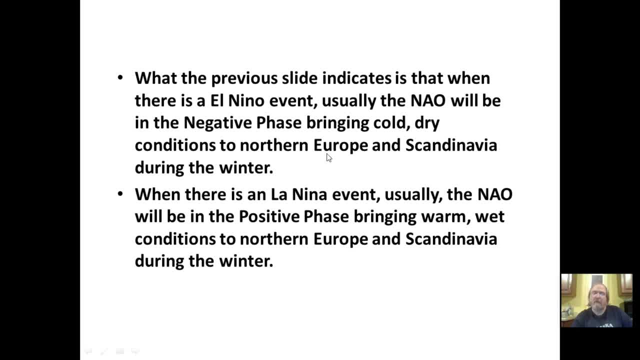 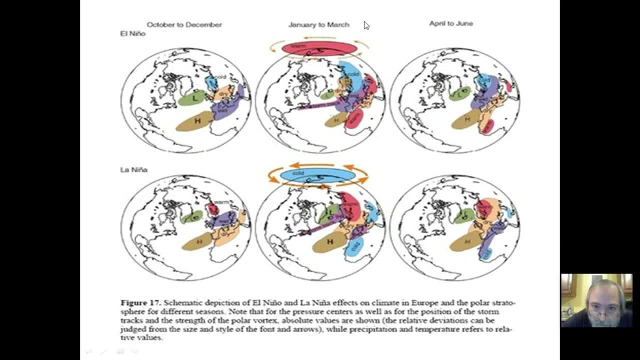 to northern europe and scandinavia during the winter. okay, that's el nino up here. now we're bringing cold, dry conditions to northern europe, right, cold dry winter, cold dry. obviously april, june is coming out of winter. so, el nino, so this top row, here we're basically. 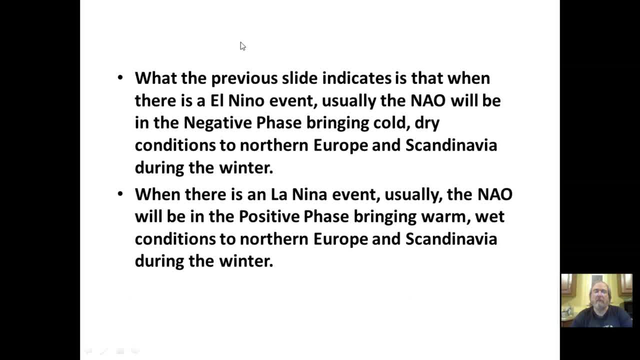 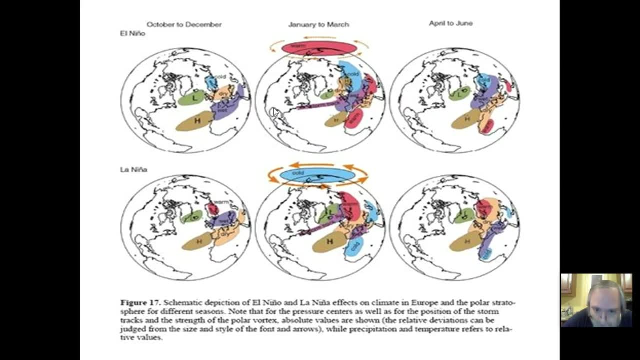 having a positive phase of the nao. when there's a la nina event, the nao- excuse me this is it- being the negative phase when there's a la nina event, the nao will be in the positive phase, bringing warm, wet conditions, northern europe and scandinavia during the winter. okay, and we can see that here. 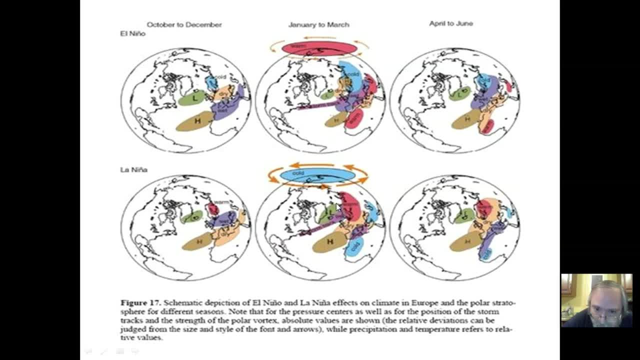 right, warm and wet right here one way. so, la nina, right, the direct storm track. so the nao is in the positive phase here, here the nao is in the negative phase here and we have cold, dry conditions. but don't forget, el nino moves eastward, the lows does, and with the teleconnection, 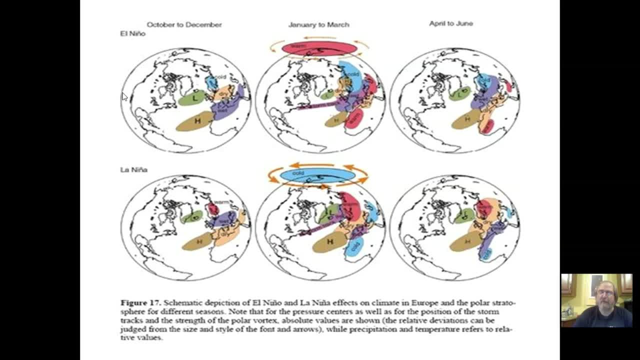 between the atmosphere and the oceans, and remember i discussed that towards the end of the uh nso video. yeah, it makes sense that there will be some connections and so there's something and they are the. then solans do have the nuna, so this is showing that uh. 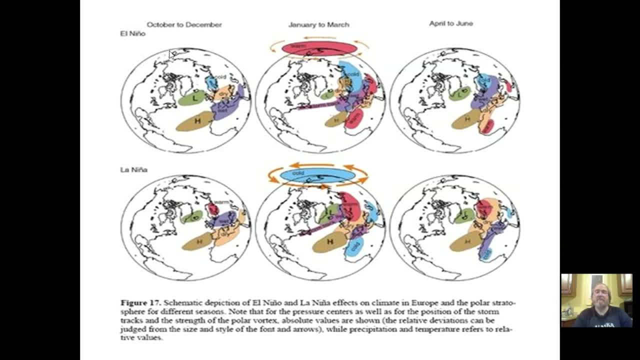 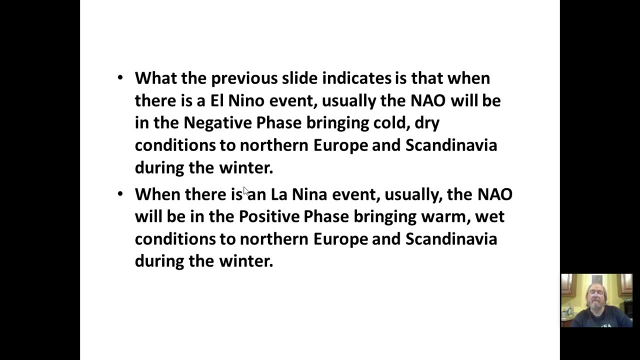 el nino is the negative phase and this is showing that the helio will respond and so forth. it's so, and so could be driving in the oh, and any of be driving, and so so this is just showing that, uh, el nino can be associated typically with the negative phase. 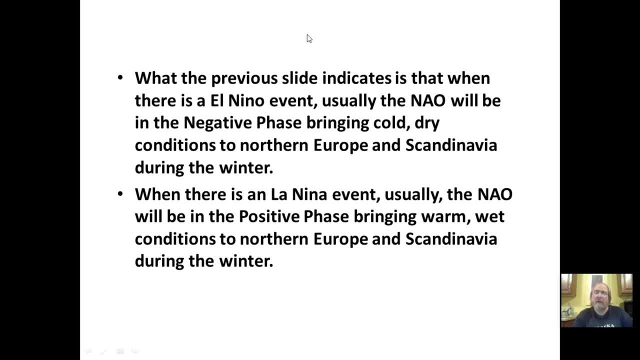 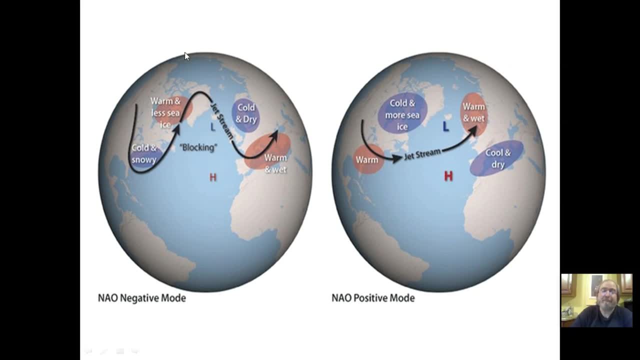 So I'll end this video here. as you just saw a sneak preview, I'm going to next do a video discussing the Arctic Oscillation. So basically, this is what we're seeing. This shows the relative strength of the pressure system and what's happening. 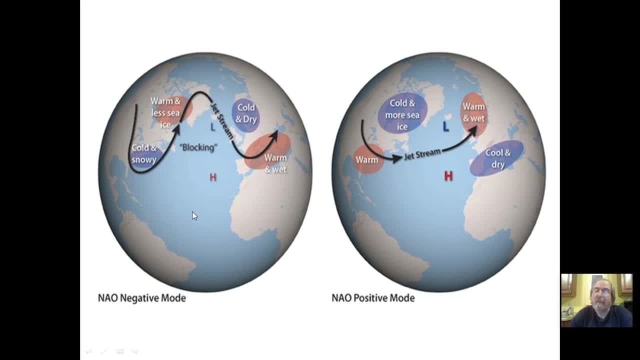 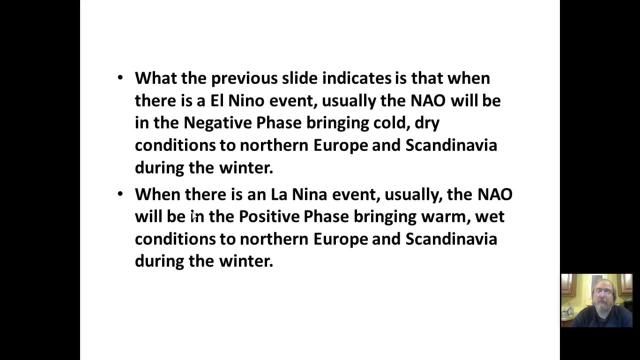 This is the negative mode, that's the positive mode, And then at the end, I showed you how it tied in to ENSO And this is the La Nina event. it's typically associated with the positive phase. The El Nino event is typically associated with the negative phase.